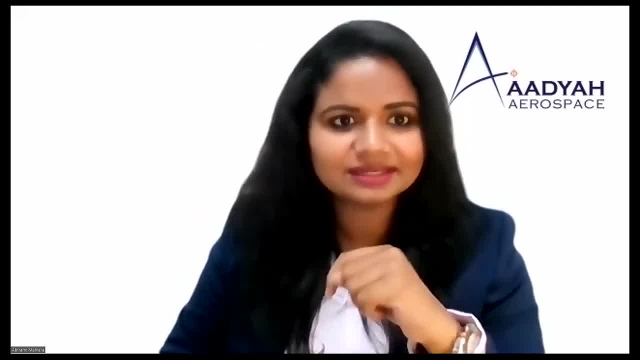 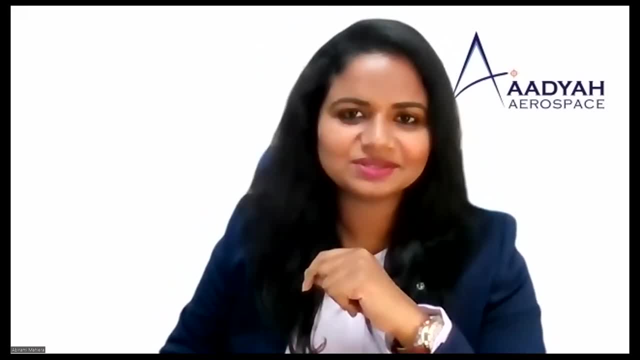 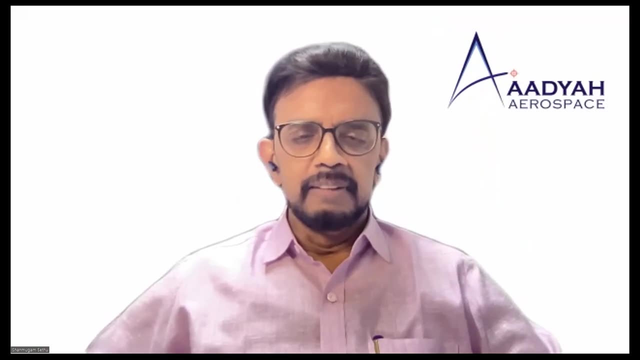 into the Q&A window you can find towards the lower end of your screen. We shall be addressing them during the Q&A. When a query is being addressed, I shall unmute the seeker for a better interaction Over to you, Mr Sethu, to lead the show. Thanks, Ibrami, and that was for the nice. 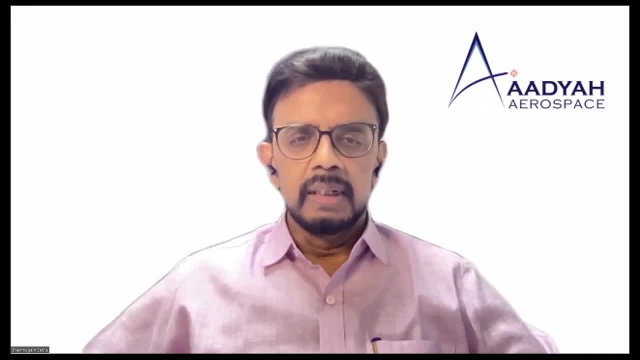 introduction and then a hearty welcome to all participants. We have an exciting evening ahead. We have put together an exciting backend space. It's always exciting, so a discussion on space will also be exciting. So, without wasting further time, let us deep dive into the presentation. 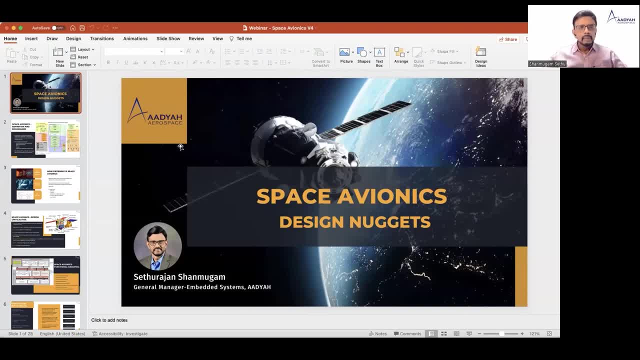 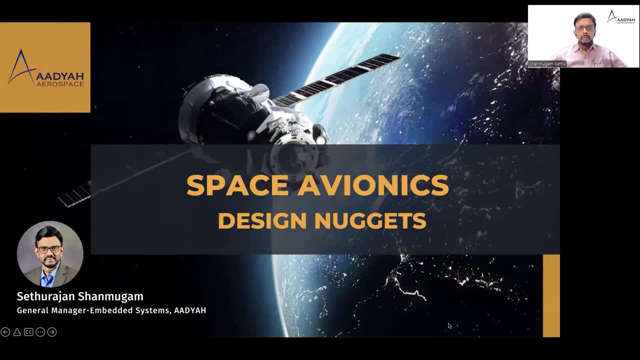 Thank you, thank you, Okay so, but the way we have organized the package for you today, this evening, is that we will give you what we what we define as the space avionics. We also give you an idea of what the face avionics rolls in a typical spacecraft. 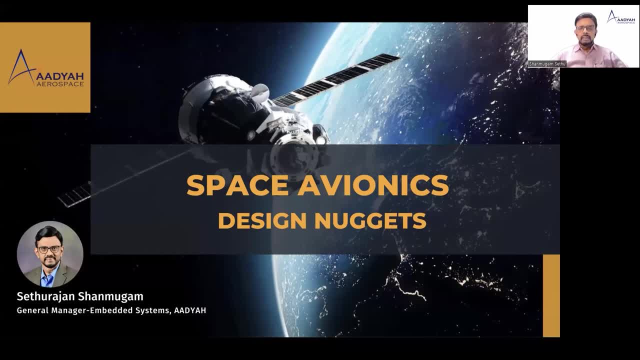 our satellite is, and we also give you the, the here list down all the challenges, what the uh avionics phase is in its operation, then we deep dive into the design and then address each one of these challenges and then we also will provide you, uh, some of the design nuggets based on the 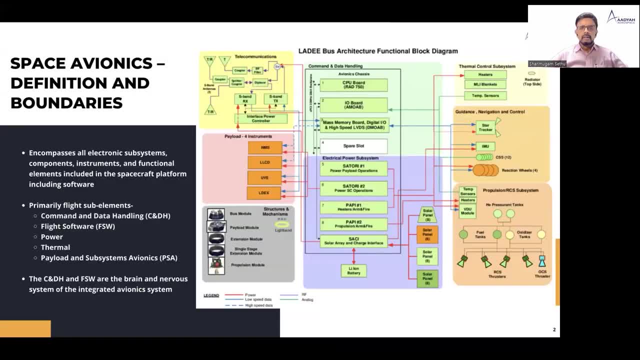 uh, our experience with the phase avionics as such. so the first and foremost is: uh, what do you mean by phase avionics? the phase avionics, in a very, very generic term, encompasses all the electronic subsystems which go on board the spacecraft or a satellite. it may be a lunar vehicle or it can. 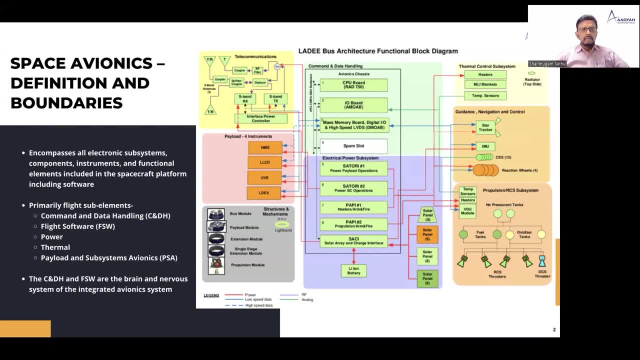 be a mass lander, but it encompasses all the electronic subsystems, components, instruments, the functional elements which are included in their base perceptor platform. now, what are these, uh components or the subsystems, wise? so the primary ones which are, uh, the first and foremost is what you call as the command and data handling. it may be a little bit, uh, unfamiliar to the 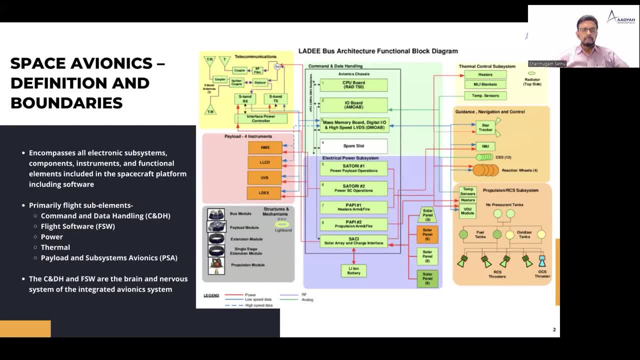 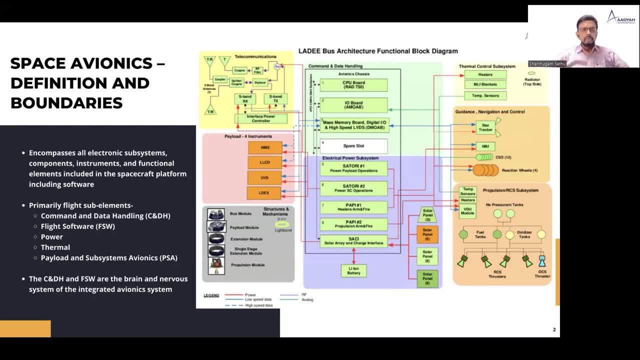 from the ground center and then it uh executes those commands and then the system also handles the data traffic between the satellite or the for the spacecraft and the ground. so that's the very much, the uh very major subsystem on both the spacecraft. obviously the software is another major component of the spacecraft subsystems. then 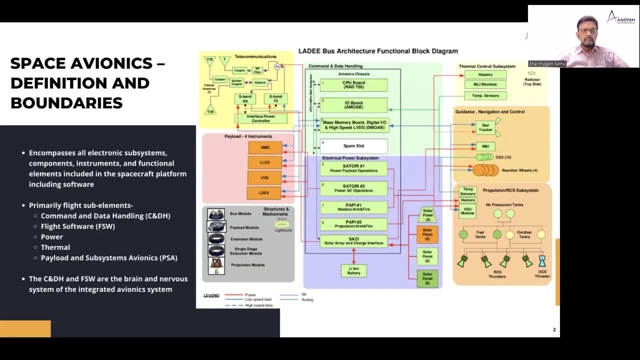 apart from the software, we have the other major systems such as the power thermal and the. of course, each mission will have a dedicated payload and the subsystems, avionics. so there is a portion of the phase avionics which is also dedicated to the payload of subsystems and avionics. 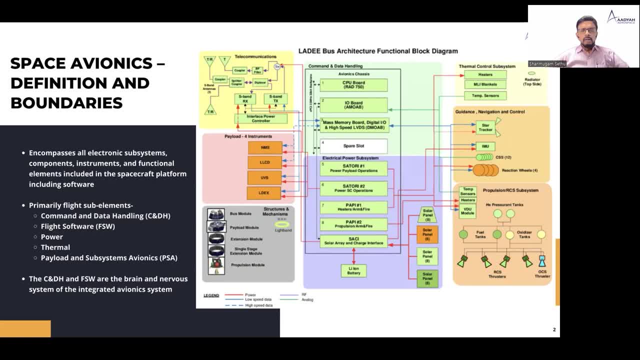 so that's uh in charted level as a psa. so the, the command and data handling, and the flight software, or we can consider it as a way over the graphic. here we have chosen the, what you call as a lunar atmosphere dust, and our environmental explorer aircraft, which 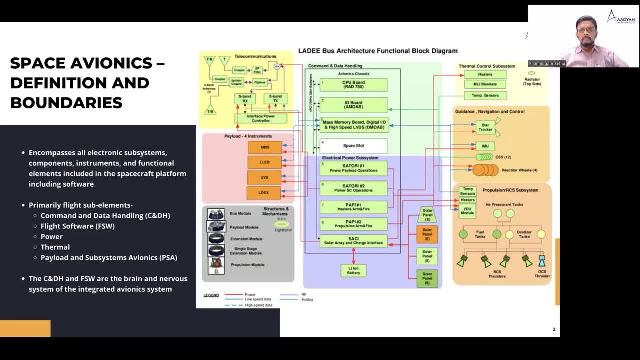 nasa has sent in 2004 and uh, as per plan, uh it uh impacted the moon. this- i choose it because it has got uh all these major subsystems, like the command and data helicopter thermal, as well, as what you find uh depicted in the graphic, is something which is not listed in my 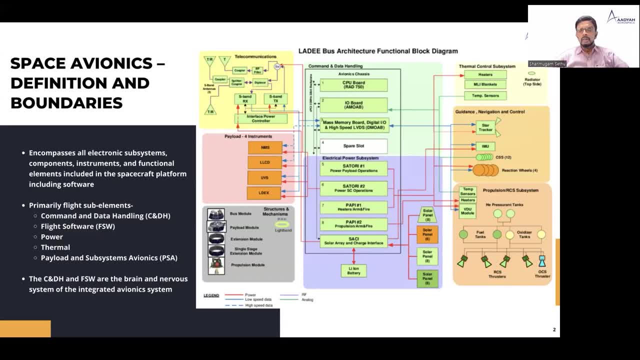 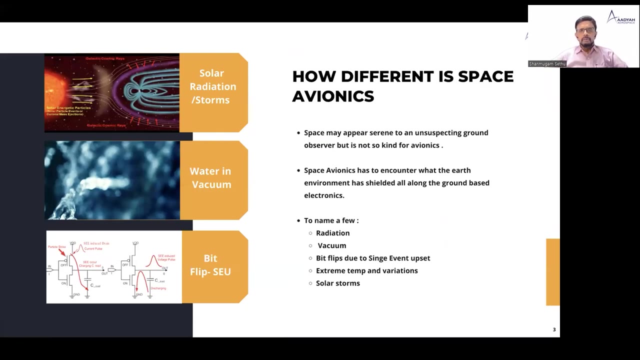 text is uh, the guidance and navigation and control, which is gnc for short. that again is uh a very, very critical component and any malfunction, the spacecraft will not reach this into the target. so with this overview, let us uh jump into the second portion of our package for this evening: why the space avionics is different from the 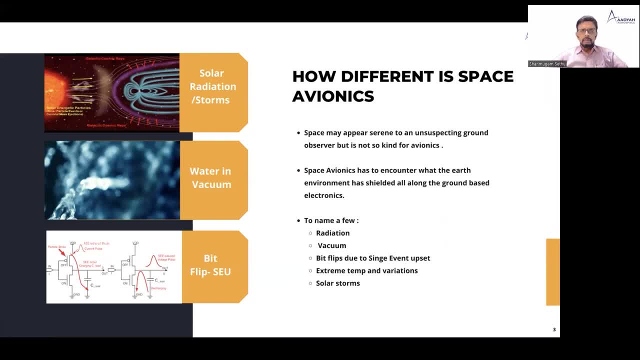 ground-based avionics or even the aerospace avionics. first and foremost is that the space is not as peaceful and serene as the seed from the ground. it is as a very, very harsh environment for the avionics, the phase avionics has to encounter. what 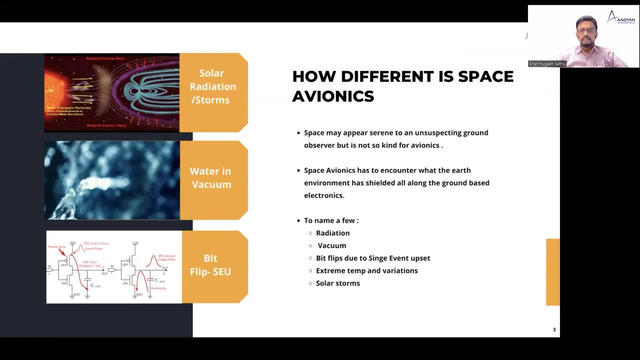 Thankfully, the nature shields us from on the earth. they have environment To start with. one of the first thing is that the radiation. The radiation comes from the solar or from it may be the cosmic rays as such, but yet the radiation what the phase avionics has to. 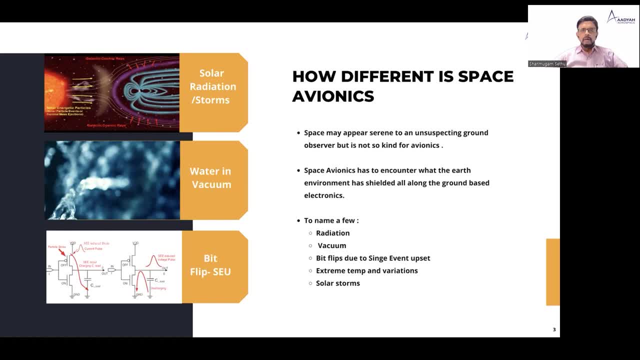 encounter during its operation is the first and foremost challenges it needs to handle it. The second challenge is the vacuum itself. So a vacuum brings its own complexity into the functioning of the normal electronics. So we will deal with detail in the subsequent slides. 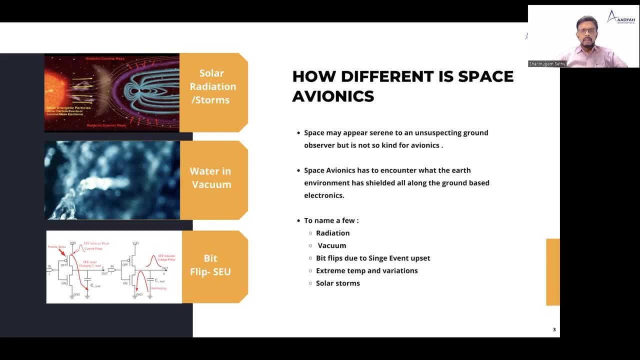 So, to summarize, radiation vacuum and then the impact of radiation, like what the single event upset, what happens in the inside, the electronics as well as the. the other factor is the extreme temperature variations which we encounter in the space, which is almost like five or ten x times what you see on the ground, on the earth. and then you also 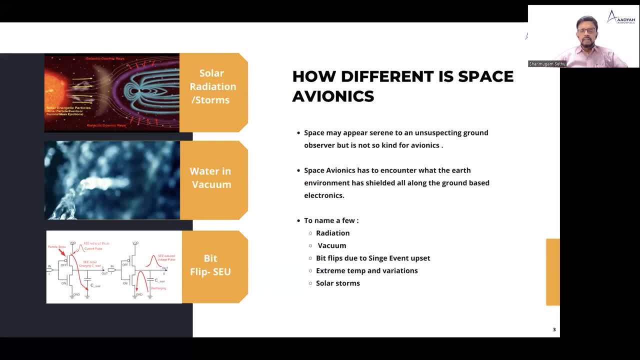 need to consider the some sort of sporadic events like a solar storms. but you could have seen how the devastating effect it can have on those spacecraft because they are almost like 40 SpaceX communication satellites that knocked off their orbit because there was a solar storm. 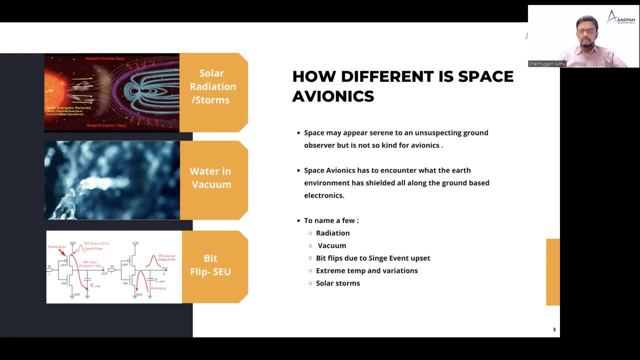 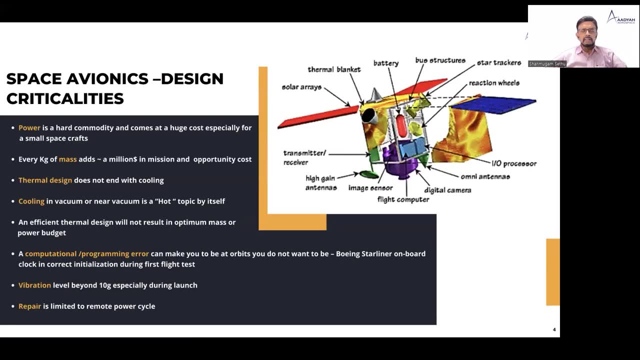 Okay, so this gives you a peek of what the avionics has to encounter in space. Now, further on to this one, what are the design criticalities which the any phase avionics developer has to address? First and foremost is something which we take for granted for the ground-based avionics. 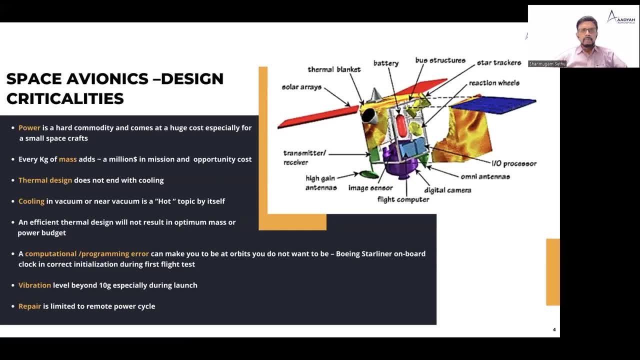 That's the power. What the designer has to keep in mind all the time is that power is a very, very hard commodity to come by and you need to plan for every milliwatt of power consumption by their their phase avionics. The second consideration, which it has to be at the 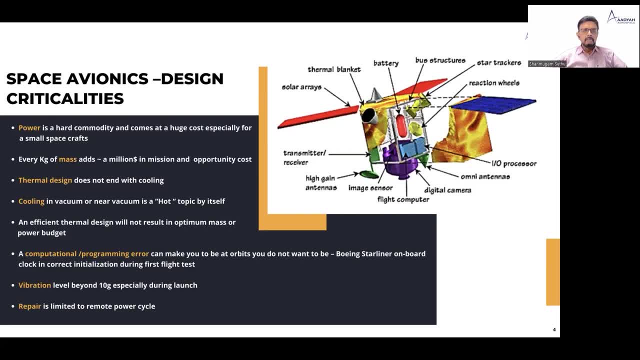 back of every phase avionic developer is the mass. A simple mathematics you can say is that every kg addition of mass in a phase mission means that you are going to lose around million dollars, either in terms of additional mission cost or the opportunity cost which you 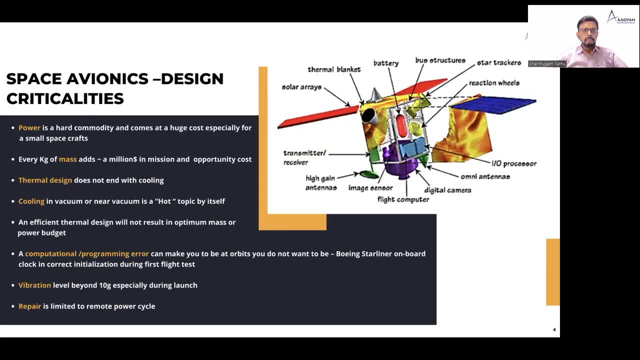 get out of carrying the additional payloads. Thermal design is much, much more complex than the ground-based avionics or even the aerospace avionics, because it doesn't end up in cooling the avionics within their operating range, but it also needs to provide for the exactly the opposite. 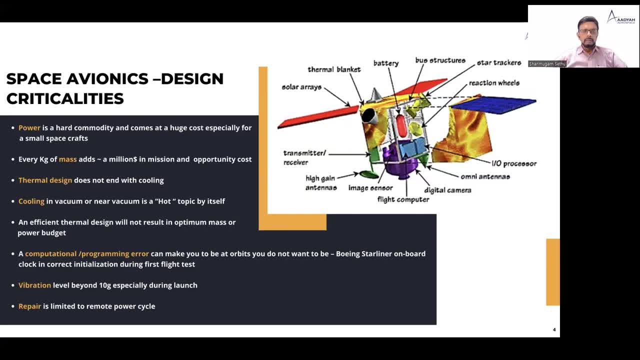 it needs to heat up the avionics, to keep it within the operational region. For example, during a lunar night, the lunar mission avionics has to be kept in its operating temperature range. Now, it is not that you can design an efficient thermal system standalone, because the moment you design a very, very super efficient thermal system. you can design a very, very super efficient thermal system. 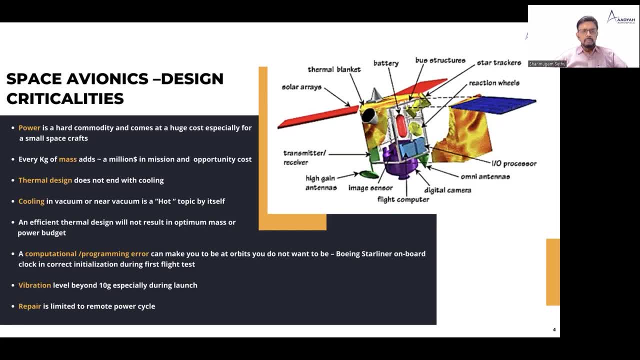 you will blow up your mass budget for the space mission, or you can. you will also end up in blowing up the power budget. So it's always a trade-off between your thermal design and the mass budget as well as the power consumption on both the missions. Then consider that the software error cannot be just. 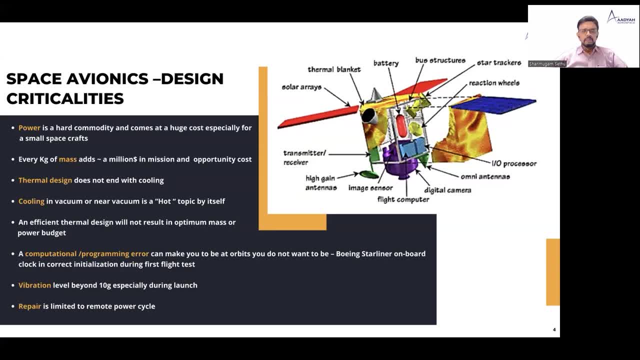 dealt with by a research team of your computers. that has its own implications on board, although a reset can still happen, but the correcting a software error is going to take you for days or months. also because the entire new software has to be applied from the ground and then it needs to be downloaded onto. 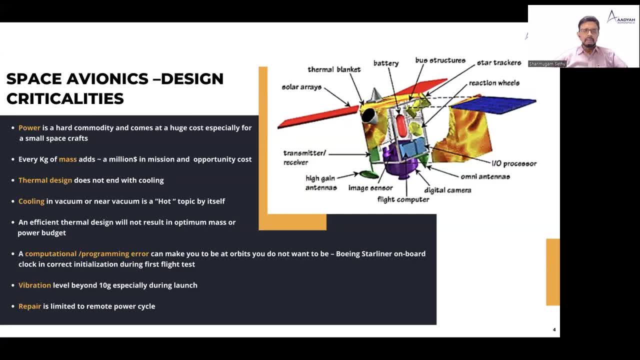 the avionics and then not that it will not happen, but you will know how much of impact it will have on the mission here simple computation error. an example recent is that, the bowling straw liner. there was a software error in initializing the onboard clock and that had a devastating effect. 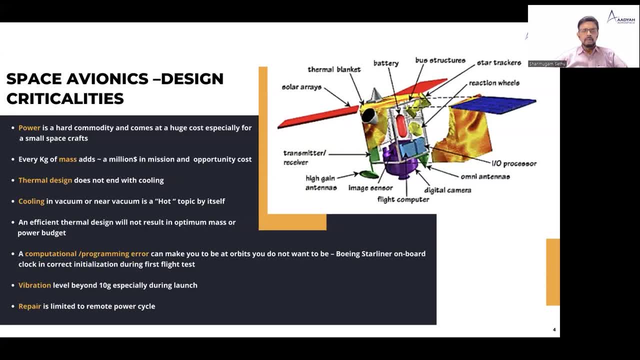 that a starliner was just meant to dock with isis never doctor diocese and the mission has to be abandoned and then had to be landed back to earth. so a simple initiation clock error can have a devastating impact on your mission. then comes, which is again a very, very specific requirement: 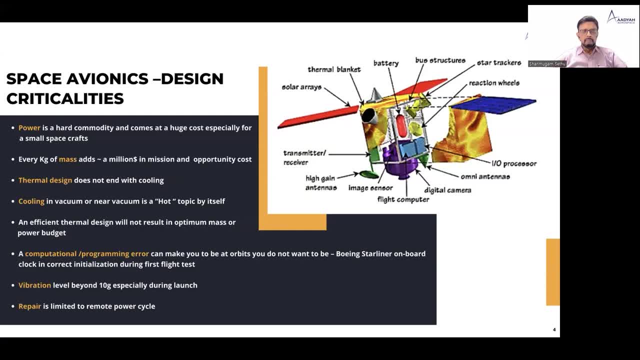 which the avionics needs to meet is the vibration level. they are much, much greater than what is specified for the ground-based electronic system or aerospace. we are typically talking about 30 g levels, as less 20 g levels, and the last and foremost is that which is like repair. 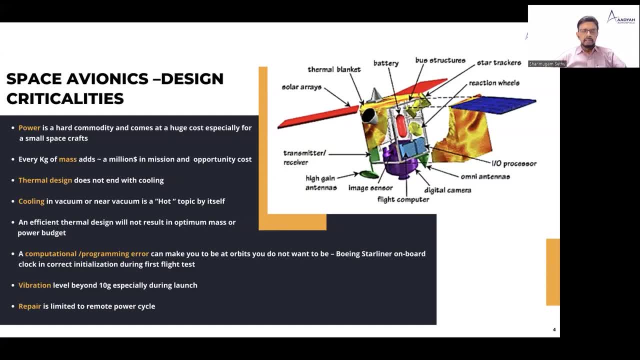 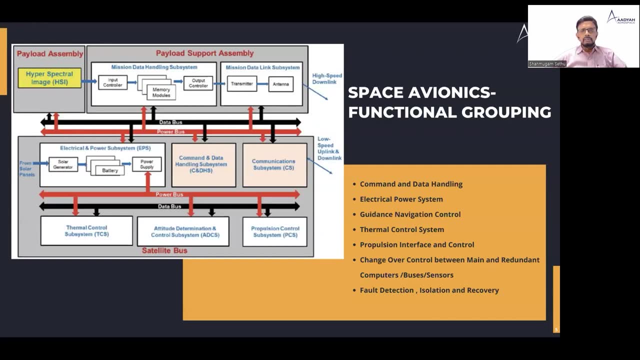 you can only repair of any mission avionics. this has to be. the only action you can do is to power cycle it and hope that it's able to come back in a healthy state. now you have here your chart which depicts it in on from a different perspective. the function, 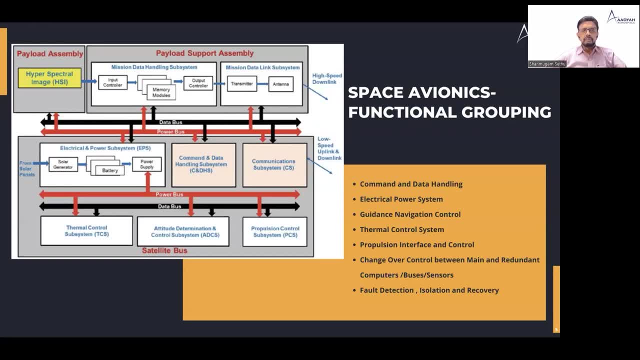 of the avionics is based on the functional grouping, that means based on the functional features of the space mission. so there again you have the commander, data handling, the electric power systems, the guidance and navigation and the thermal control systems propulsion interface. now let me spend some time on the proportion interface, which i have listed down for the first. 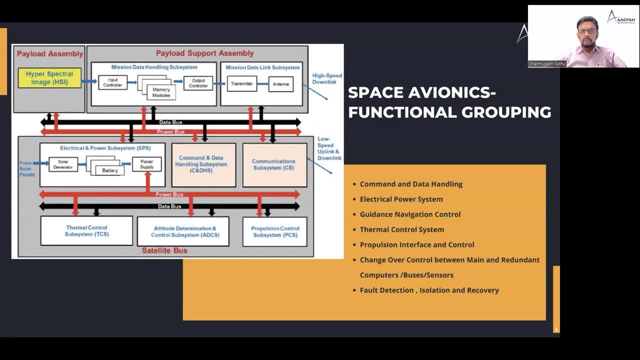 time in this representation, the propulsion interface and control. avionics is the link between the computers and the propulsion system, consisting of the thrusters or the reaction control systems which are makes the maneuvering the spacecraft in or the satellite in space. so it's, so it has a unique function, that it has to be the single point interface between the avionics. 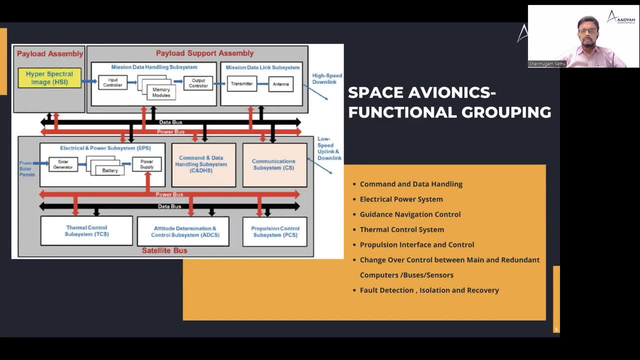 and although it is also part of the avionics, but also it is one which is going to command and then the propulsion system and get their feedback. incidentally, i should mention that adia is currently executing a program for a singapore based customer for exactly for this propulsion interface and control system. apart from the other. 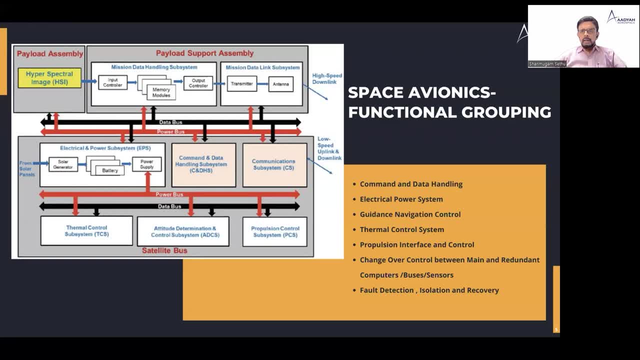 aerospace program which i've already mentioned, though i've also specifically mentioned the other piece of avionics which is like quality is a changeable control between the main and redundant computer buses of the senses on both, uh, the spacecraft phase avionics. now you may wonder why this requires a special mention. 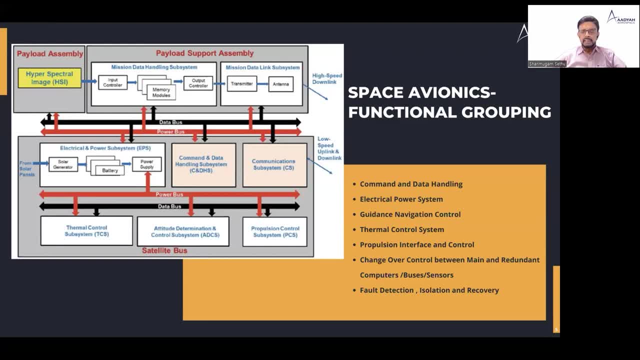 because sometimes it will become a make or break between a mission success, because you need to execute a successful changeover. either it may be between the main internet computers, it can be between the main and different buses, or it can be between a main and different sensors, like 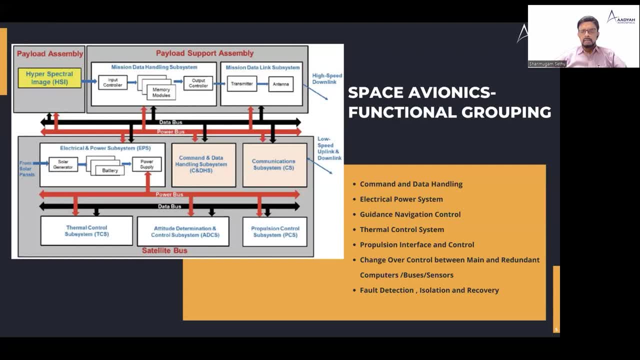 for example, there may be two main uh imu, or initial motion unit, or a secondary or a backup imu. so one of our failure mode occurs in the primary unit of any of this. then there has to be a successful changeover. the next result of uh, what i have listed over there, is the one which almost 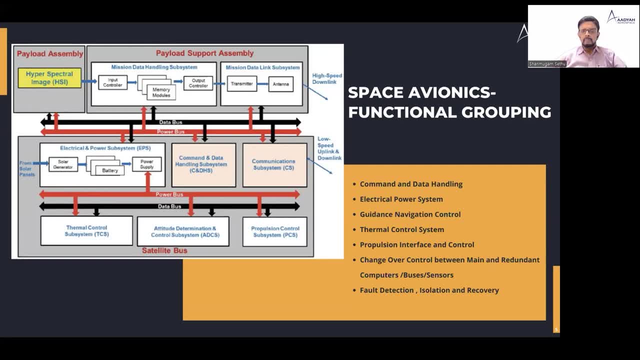 uh affects. what is this? uh, effective changeover. that means there is a piece of software on board which we call it as a fault detection, isolation and recovery, or ftir by the current images commonly known across the face of the mind. that is again a very, very critical. 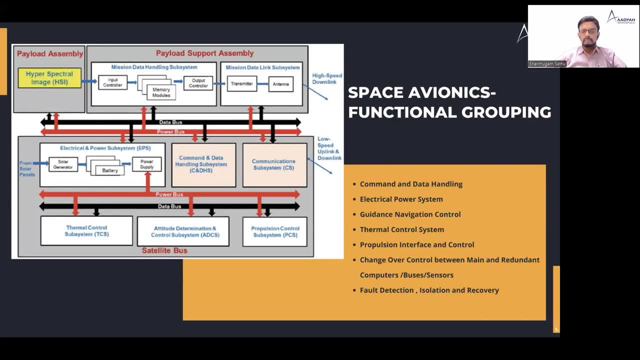 one to consider when looking at new technologies which need to function all the time, taking care of the failure modes which occur and then do the isolation and the recovery in time, and some of these recovery actions. uh, please keep in bear in mind that that can have to flow from ground also. 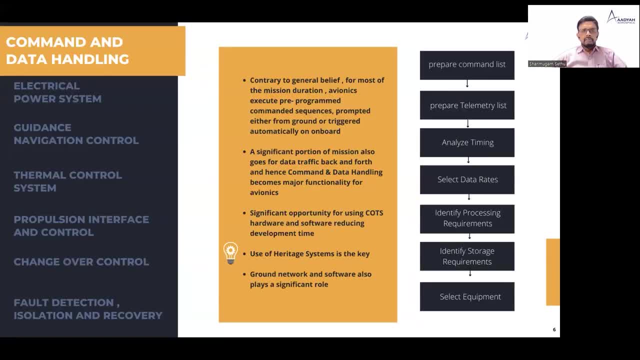 and some of them need to be taken by the onboard avionic system itself. The systems we have seen one, the commander data handling. I have described them in detail, but let me concentrate on the what's the design nuggets, what we can focus upon this chart. 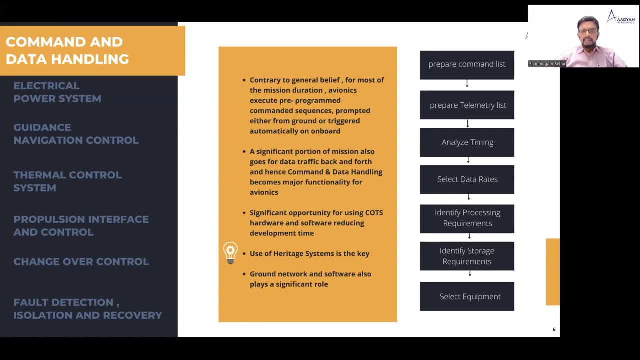 The use of the systems is the key for you to have a real, optimum commander data handling, because when you start designing the commander data handling for your specific mission, sometimes you may end up in the whole design or the design with. both are costly as well as the mission success is concerned. 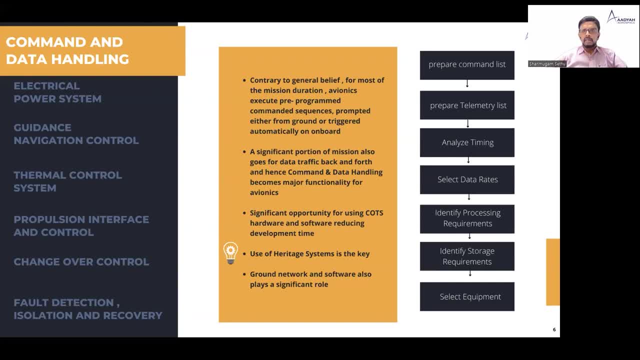 Now, over the right hand side of the chart, you have a simple flow chart. Here you are depicting the major steps for the design of the command handling system. Obviously, the commands which need to handle comes to the top of the list, And then you also need to take care of the telemetry. then you need to decide what's the data rate and then you need to decide how much is the processing requirements. 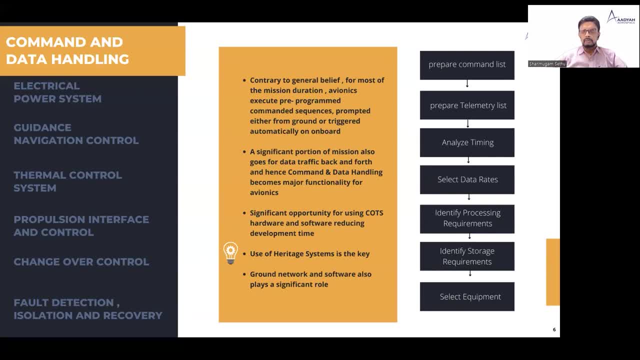 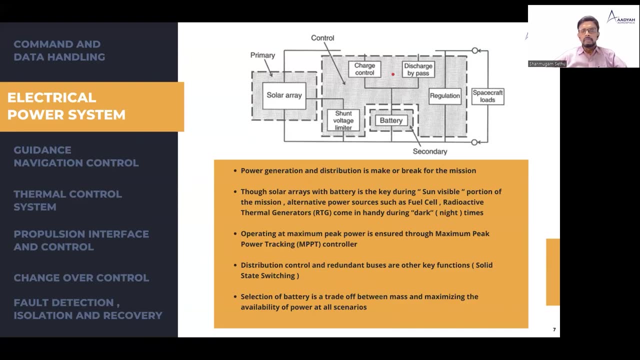 Then you also need to understand because the data though we also need to consider the storage requirements for that. With that you can zero in upon Your command and data handling system itself. Other major subsystem, as I mentioned before, is the electrical power system. 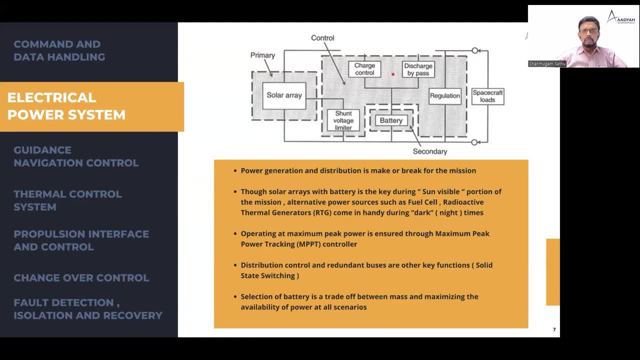 Here again, it's a common knowledge that the solar arrays will be the main component or the main power generation of onboard the phase card mission. Then you have the battery as a backup, But the control is a little bit too sophisticated, because it's not that you can have a rudimentary solar array. 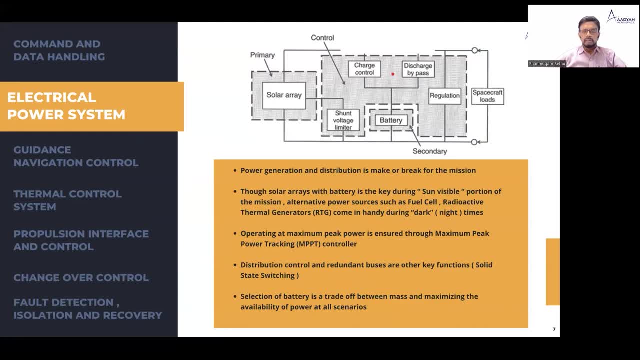 But the control is a little bit too sophisticated, because it's not that you can have a rudimentary solar array. All the power charging the battery has, the less applying the loads. They also need to be. They also need to be. there has to be a efficient point of operation. 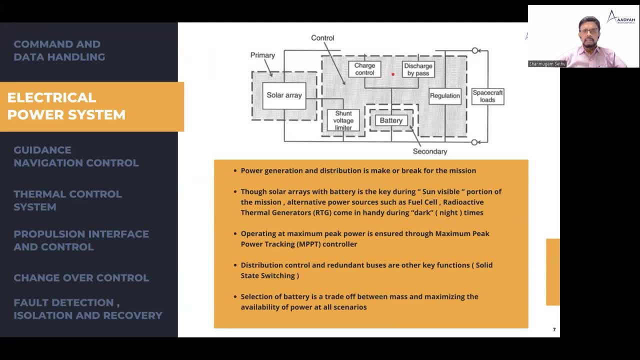 So that sort of control, we call it just the maximum power tracking control, which is always nice that your solar array, as a lesser battery charging, is kept at this maximum point of operation. So that sort of control, we call it just the maximum power tracking control, which always is that you have siloed already as lesser battery charging, it's kept at this maximum point of operation. 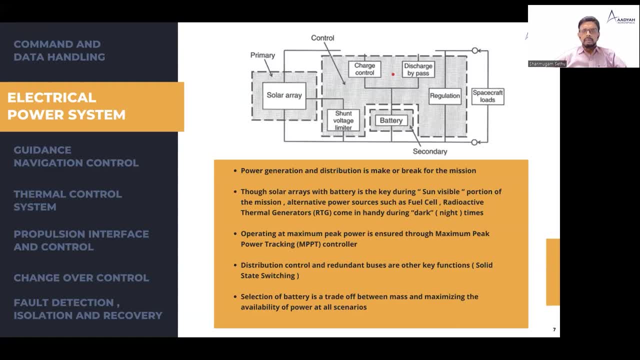 requirements for the components of the subsystem on board the aircraft. You need to design an efficient distribution system, along with its safety, as well as protections incorporated, including the power current or isolation in case of a fault, as well as we also need to take care. 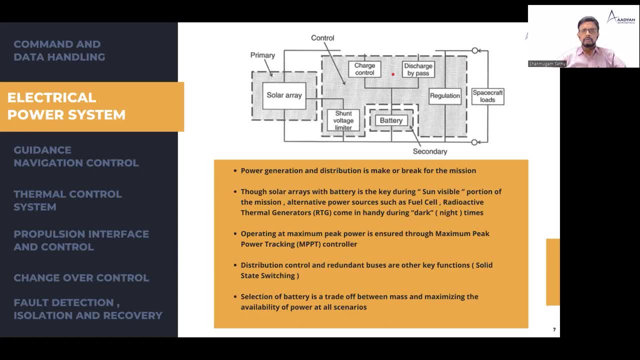 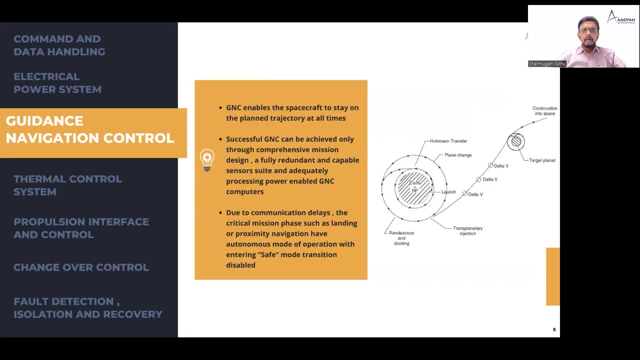 of some extreme situations, when you don't have adequate power generation. We also need to go into what you call as a selective power, off of the and maintaining only the critical system, which are required for the continuity of the space mission itself: Guidance and navigation. 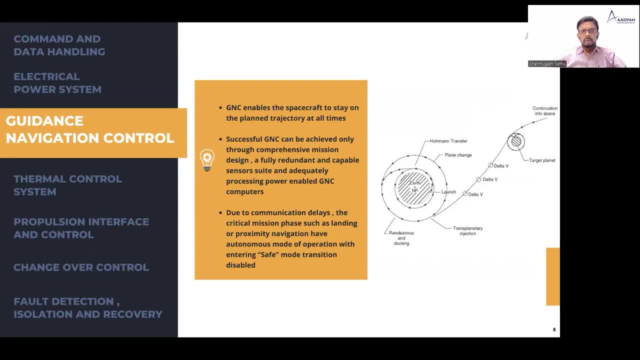 system. this is the system which guides, which takes the aircraft spacecraft to its final destination. Now, this is a pure- I would say this is a pure art and science, because most of it is again driven by the our mathematical computations of the forces. what acts upon the spacecraft? 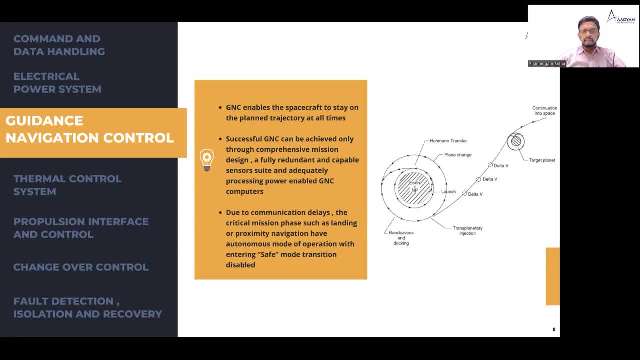 And it's a quite a bit of elaborate exercise, which starts with your mission planning And then you need to match the your maneuvers with the propulsion system capabilities that are depicted in the chart. That's delta V, delta V that we import. 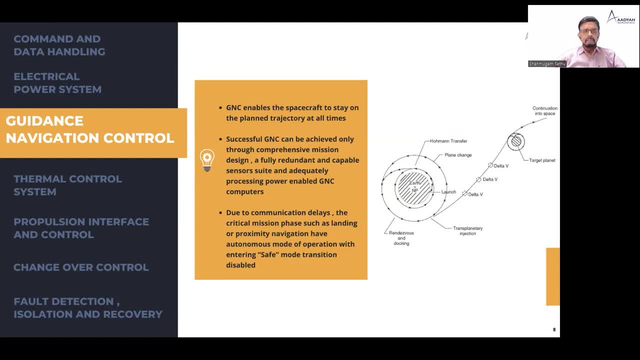 Yeah, Delta to the velocity of the spacecraft. So, and other thing is that, um, not all the times this will be effected from the ground. There are some phases of the mission where the guidance and navigation needs to be happening autonomously. Yep, The famous example will be when there is a 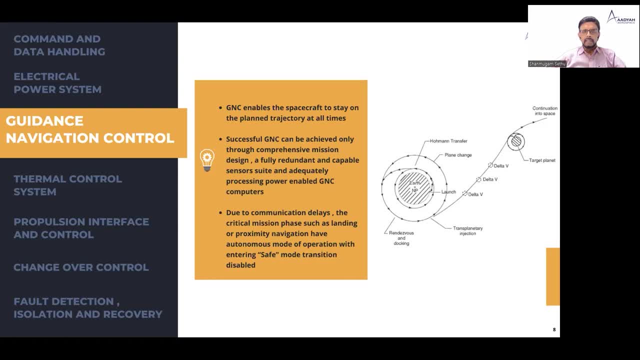 landing phase in a planetary mission or interplanet mission. there, uh, there's always- I don't know one of the speeds that you're on, So usually there is not, unless you have a ship based on the ground When you're in the area, the land side airspace for, for example, and there are, you know, there are. there are active active active, active active land space. If there are not, if there are active airspace, there are multiple spaces and then there's airspace When, if you uh, there are. if there are not, if you uh, there are. if there are. 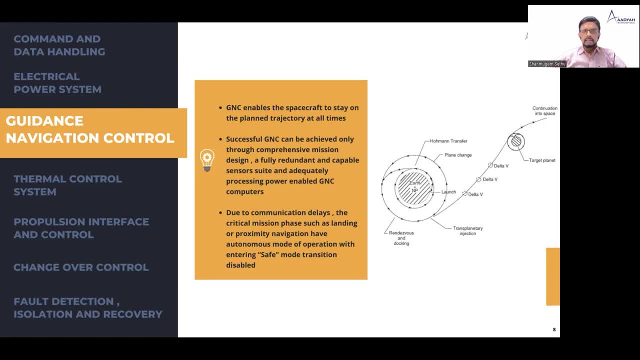 your time. criticality associated with any landing and the delay between the communication between your earth and the ground will not enable your ground-based GNCT to operate. so the spacecraft into what you call as the autonomous mode, where the entire software take care is operated autonomously by the spacecraft itself or to ensure a safe landing and during autonomous 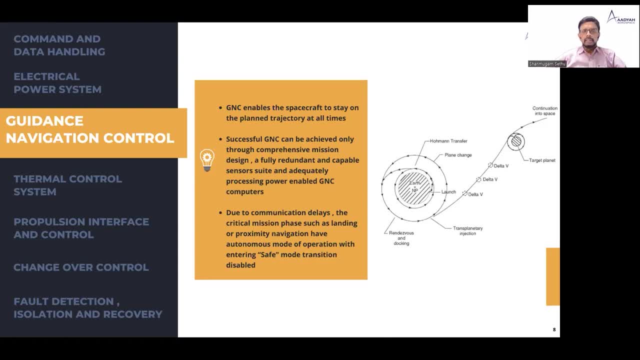 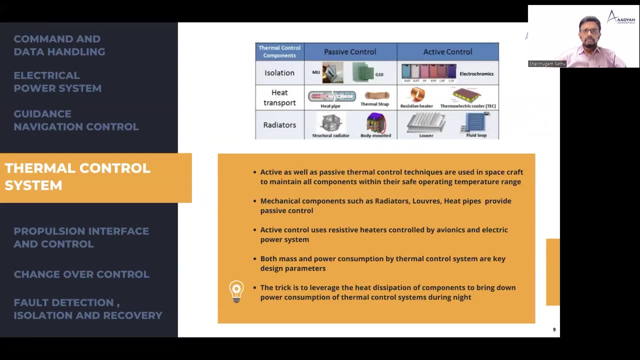 mode. we even don't allow anything, any other change of the mode, even the safe mode of operation which is valid for the other modern phases, may not be permitted during this autonomous mode of operation without. let us jump into the thermal control system. it is not as simple as you see. 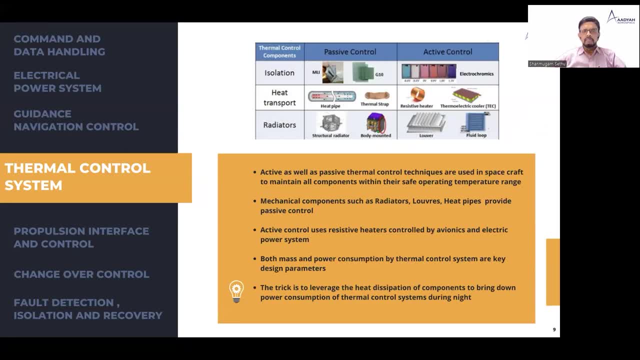 in a ground-based avionic system. here we need to take care of two things. one is we need to isolate the subsystems from either the extreme cold or the extreme hot, so the isolation comes with the top functionality of the system. then we need to transport the heat either. we need to transport it. 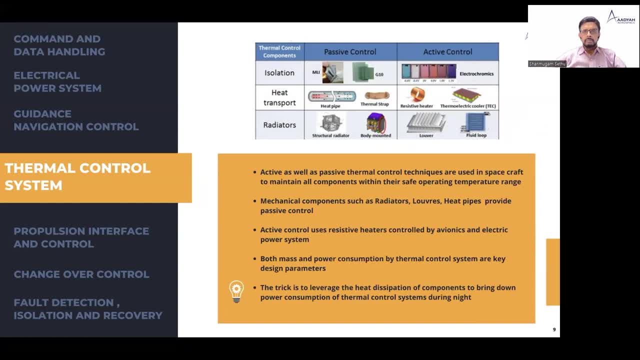 out of the system or we need to transport it into the system to keep it warm. then comes the radiators or dissipate the excess heat as such. so this itself is a science, and then there's always a very, very technology intensive system where every now and then there is always a 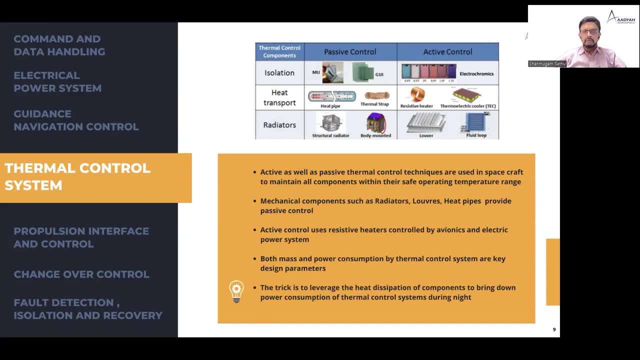 efficient way of encoding. again, the mass considerations also drives the development. now the design nugget is that suppose you are designing your thermal control, your sun absent or do not light operation, the. the trick is that you liberate the normal heat dissipation of avionics and try to minimize the excess heating required. 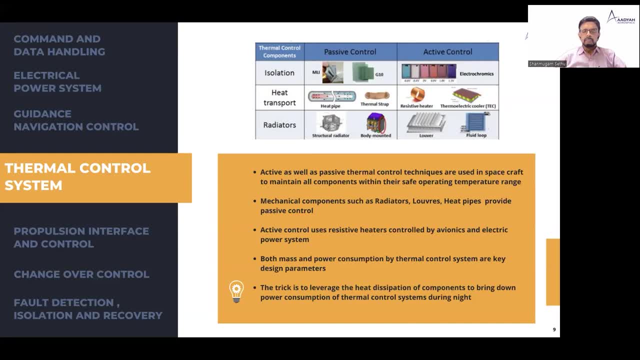 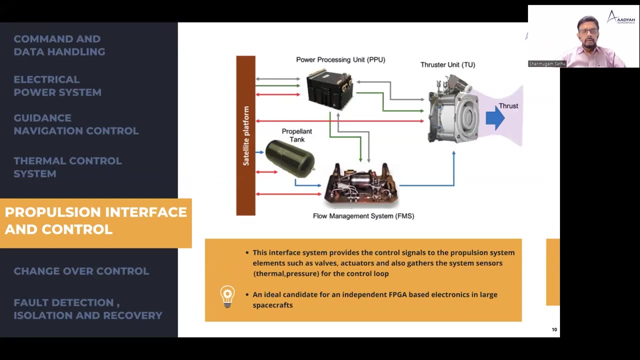 to keep the avionics in itself. i think within this about the cold out environment temperature- and bring it within the operating minimum limit, such This I talked about before and then, so I will quickly go over and concentrate on the, which is the design nugget over here. 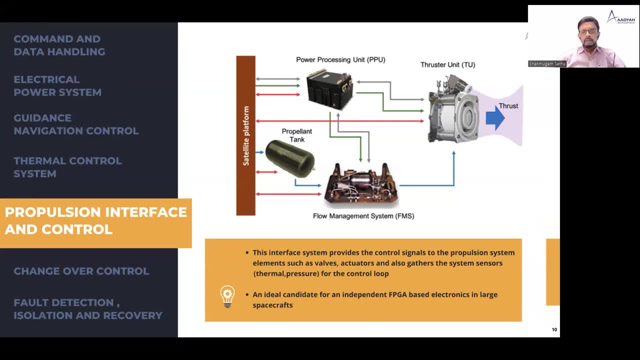 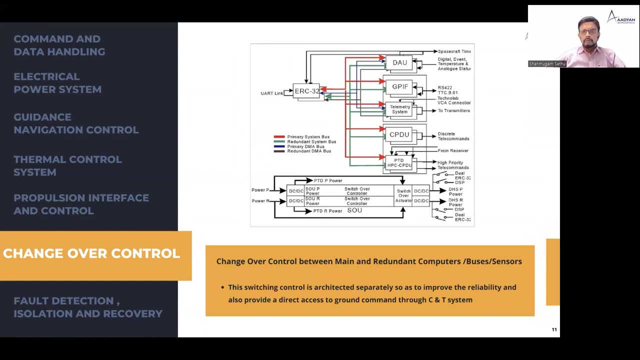 This system being a link between the other computers and the propulsion system, there is an ideal candidate where we can try to bring in some efficiency by having the implementation through an FPGA, So with that we can move over to the other portions: the changeover control between the 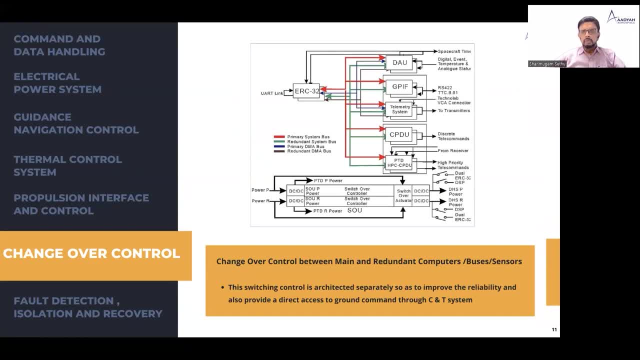 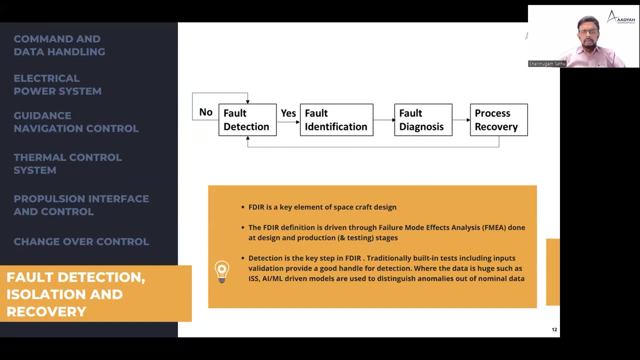 main end residence. and then we also need to ensure that this changeover takes place on time so that we don't have impact on the mission success of the mission as such. This I talked about, So let me focus again On the are design negative here now, the first and foremost, the successful fault detection is 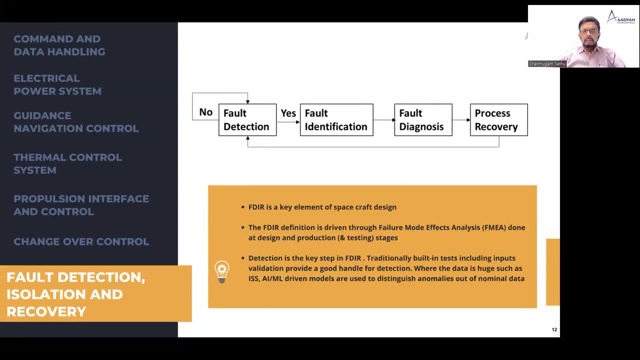 how do you detect the fault? that's it. that means you need to detect the fault or the failure scenario in time and then, if there are further steps like the isolation and recovery, can follow. but the detection is a key step in the fdar and the initial or traditionally the 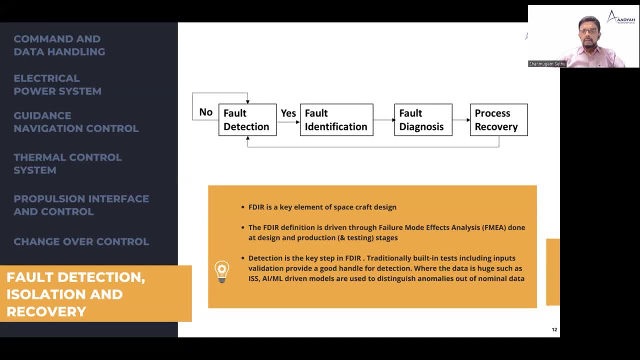 fdas used to be based on the built-in test already based on the, the models of the subsystem running inside the software. now, awfully, there will be now a push towards the use of the ai. that means the, a models which are you prepre, pre-programmed or allow them to learn from the nominal and the 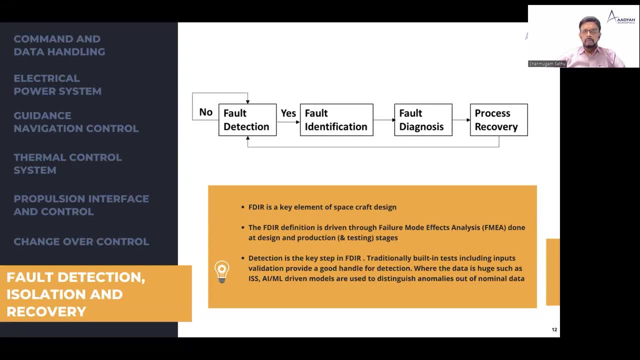 fault, failure data. so you have the model, and then the model operates within the onboard software and then makes the efficient detection of the software. this is supposed to be more processing wise. it is supposed to be more efficient than the traditional models running, or even the bytes and other. 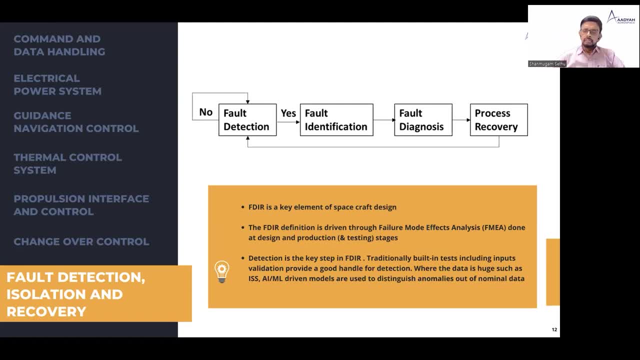 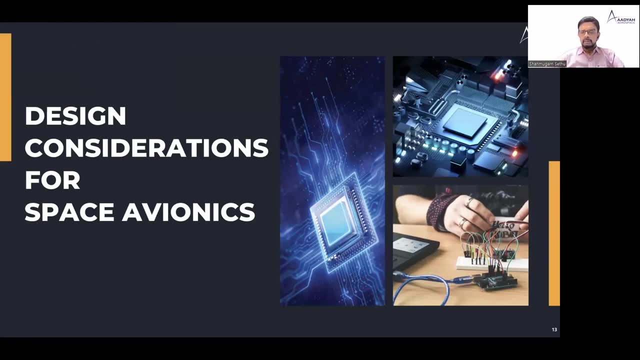 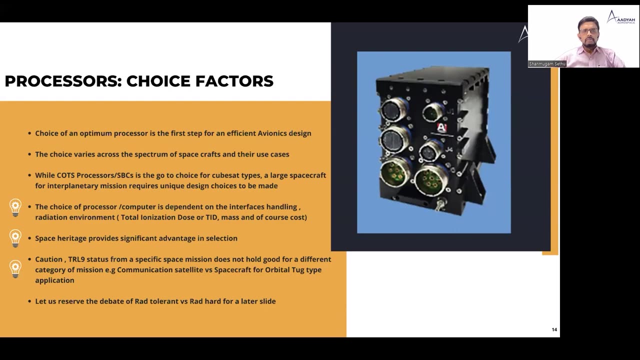 ones, which also consumes much of your execution time as well. okay, now coming to the main topic of the for that uh this evening, which is the design considerations for the base avionics. first and foremost uh is to address the first and foremost challenge, which is the uh, uh, the uh. 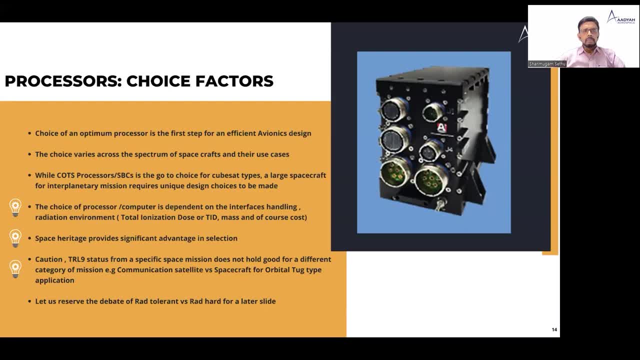 in the in any immune design, the choice of the optimum processor almost ensures that you have uh ensured a good probability for success or the safe operation of the avionics. but um, for the phase avionics, the uh, the environment causes its own challenges with respect to the choice of the processor, whereas on the ground-based avionics it will be based on much. 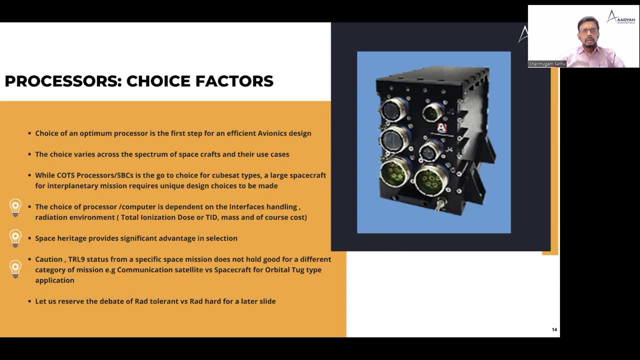 much more avionic characteristics, like: what's the uh processing capacity required, what's the memory capacity required, uh, what's the um? probably uh, the uh, uh, the response of the system, both in uh temporal as well as the space domain. so all these considerations, which are the traditional ones, 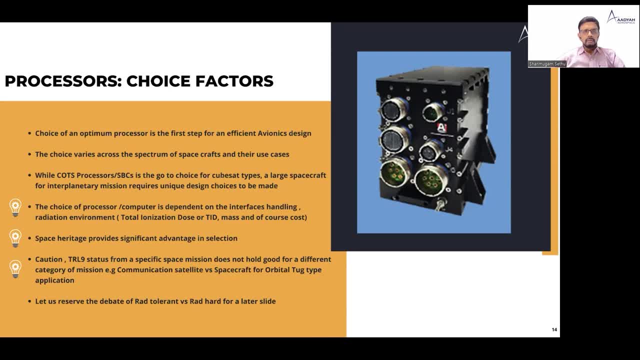 which goes into the choice of the processor, is a little bit uh complicated to the phase, because there is another factor coming in which is the radiation information environment. now your uh um choice of the processor may be from the radiation environment, because it is not the uh. you are going to change the processor, but you need to change the type of the processor, whether 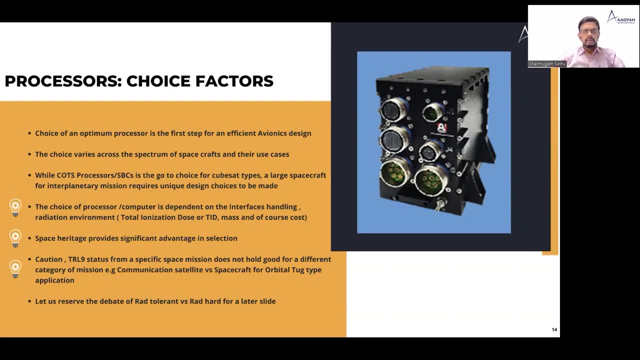 you want a radiation hardened processor or a processor which is going to tolerate the radiation, or you can go in with the other protection for the radiation in your normal processor. so this decision now is shifting to the environment rather than the avionic characteristics. there are some parameters on which you can. 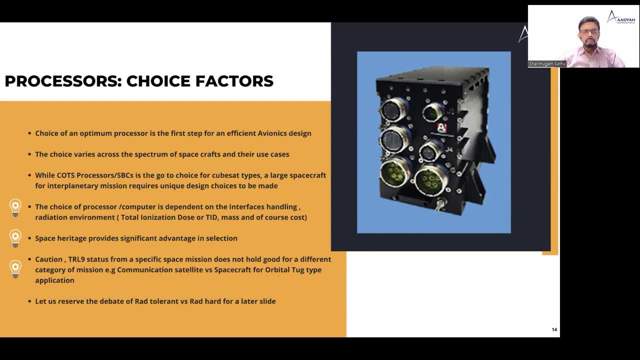 try to gauge the radiation environment. one major parameter that is used is the total ionization dose to which the avionics will be exposed during the mission. Of course, the mass and the cost is also another key factor in your selection of the processor. Now again, if you are able to, 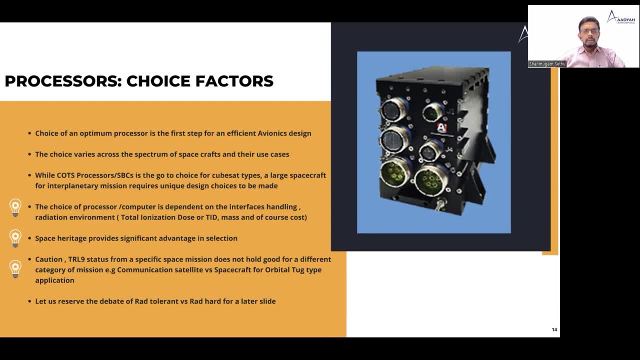 zero in on the processor which has been flown previously and then that we call it as a space heritage processor. that will give you a good heads up into implementation of the avionics or the development of avionics. There's a bit of caution around. there is that you may have located. 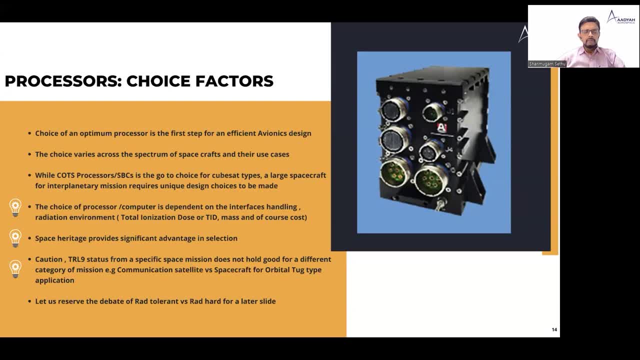 a space heritage or a technology that is not yet available. You may have a technology radiation level 9 processor, but the same. what you need to notice is that a tier 9 processor for a lunar orbital type of mission may not hold the same tier or may not. 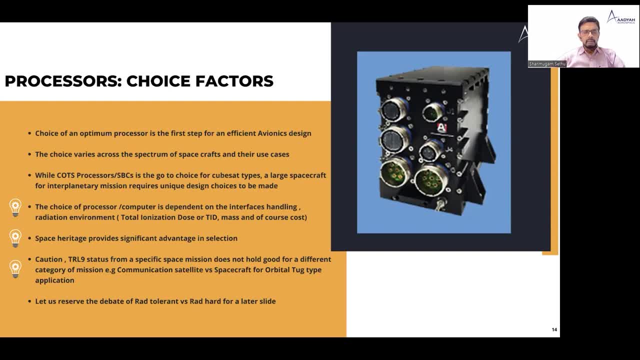 be qualified at the same technology radiation level for a lunar landing mission just because the type of mission is different. So you need to be extra careful in selecting your heritage system and don't go by the generic tag. You need to see whether the tier line is for a similar mission to yours. as such, 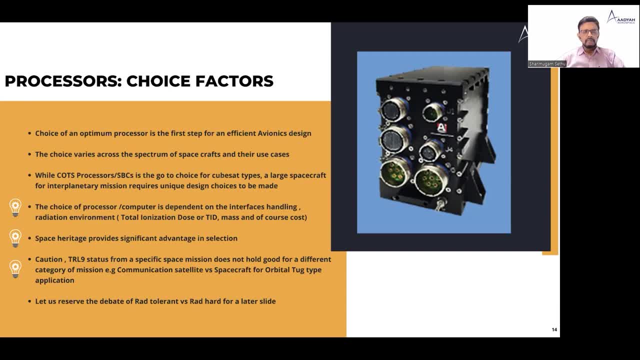 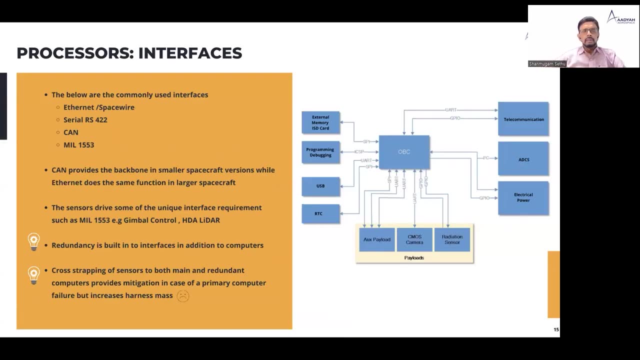 Now I will. we have further slides where we deal with the choice whether we need to go in for a radiation hardened or a radiation tolerant processor. Now a little bit about the interfaces. what the processor need to cater to First and foremost is: you do have an ethernet or you have a space wire, type of which is a. 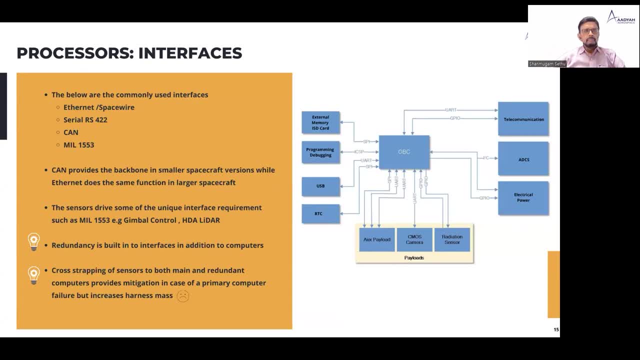 space twin of the land-based internet And you have the normal serial interface. it can be RS-432 or RS-485, or 232 is also used. CAN is gaining coinage in the sense that these can be used in the case of a large satellite. so it can be very much. 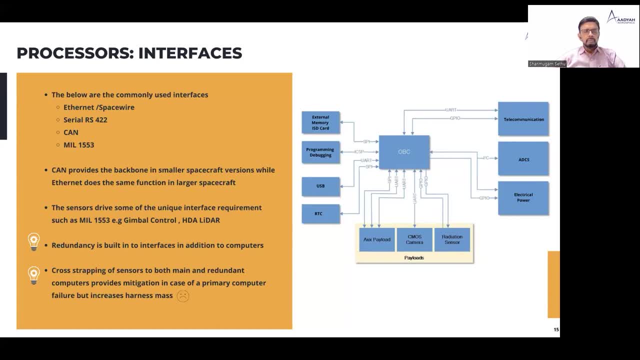 in the small space, you know, and you can have multiple levels of intensity. So if the device is very large and there is a constant auto-reaction, you can have multiple levels of intensity in the middle of the surface, such as a satellite. 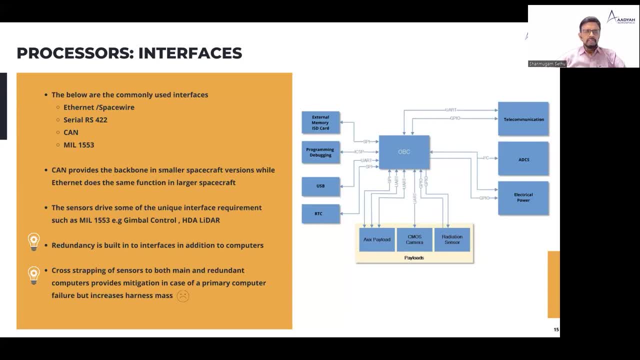 or a SMAS-type satellite And you have the Sss-2 SCT or an SST-2 SST-2, which is basically a-zero-satellite, and the mini-satellites, the smaller spacecraft and cube satellites. as well as the cost you need to pay, 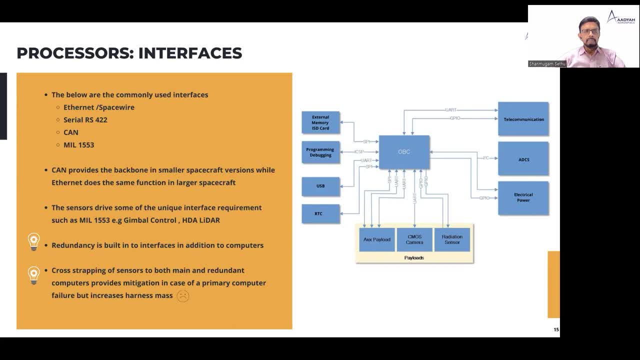 for providing the BIL 1553 interface into your computer And the design nuggets-wise. first and foremost is that we need to have the redundancy built into the critical interfaces. providing redundancy with the computers is not going to ensure you that you have an effective recovery action. 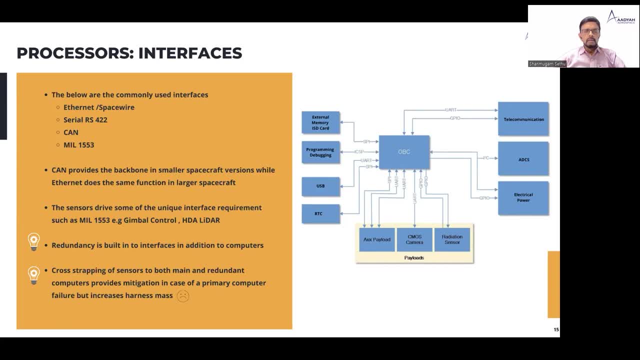 in terms of, for example, if you decide to go in with one single IMU for your mission, there is enough possibility that the IMU go out of calibration or become there. a cumulative error drives it out into the invalid range. So if you have a single IMU, 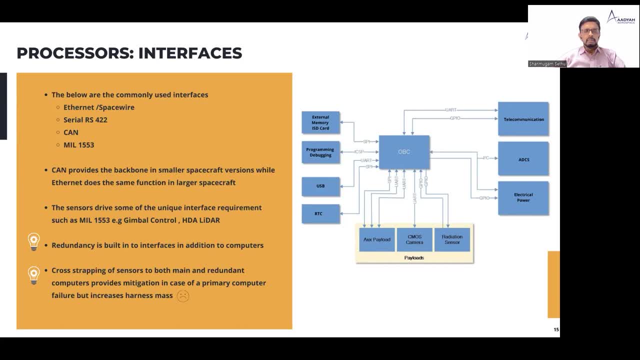 then you have to go out of the range and you are down to see whether we can successfully accomplish the mission goals with other sensors you have on the mission, or sometimes it may end up in a mission failure, like what happened in case of the Bashir Israeli lunar lander. 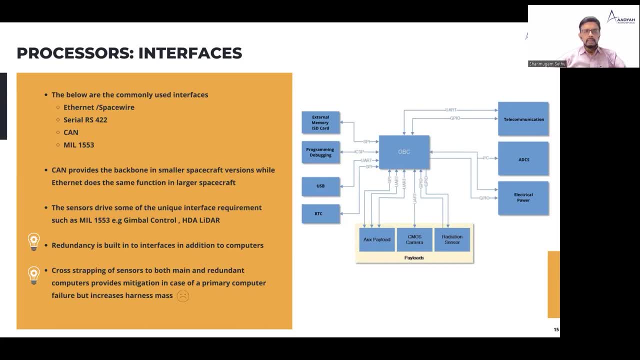 They had ran into a problem with the IMU and then they tried to restart the computers. by the time the recovery action was two, two slow and then they crash: landed on the moon. The other thing is that for providing redundancy for the sensors. 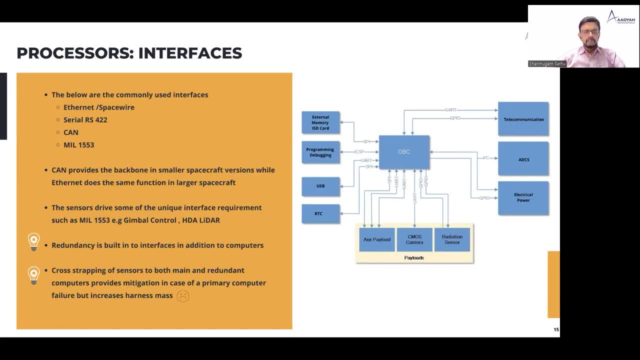 so the immediate tendency of any developer is that wherever the sensors can be crash, scrapped to be in the processor, we can do that one. But remember that you are adding to the mass and sometimes the additional hardness required. you may as well put in additional low cost sensors. 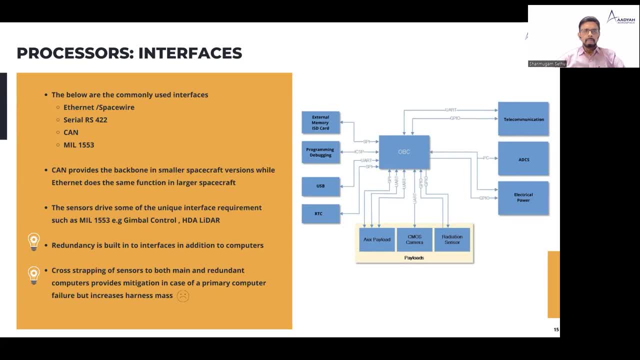 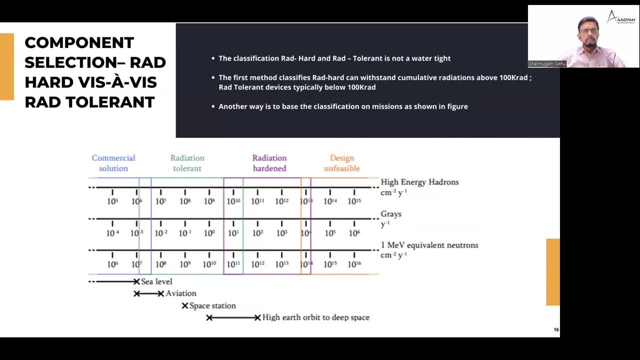 rather than cross-dropping between the computers. Now comes the what the discussion I have promised with what is the design considerations you need to make when you have to decide whether you're going for a radiation hardened component or a radiation tolerant component. First of all, the definition between these two is not very 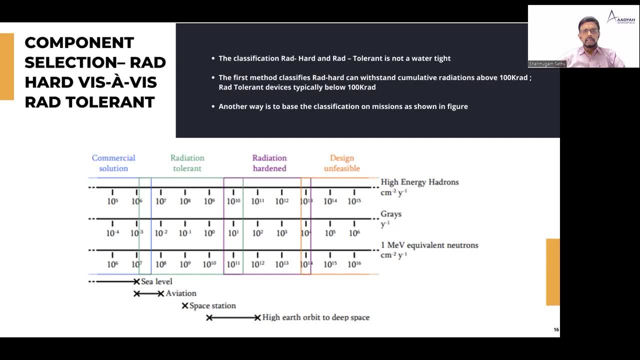 very, very watertight or very, very clearly defined. There is one definition going by the amount of radiation in terms of the kilo rad or CR, the avionics they're supposed to, And that definition says that anything about any device. 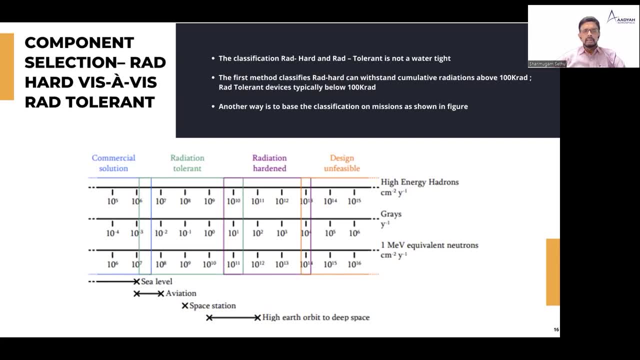 which can tolerate about 10 kilo rad will be considered as a radiation hardened device, and anything below a hundred kilo rad, which is normally in the range of 50, to 80 kilo rad, can be a radiation tolerant, And sometimes it can be. 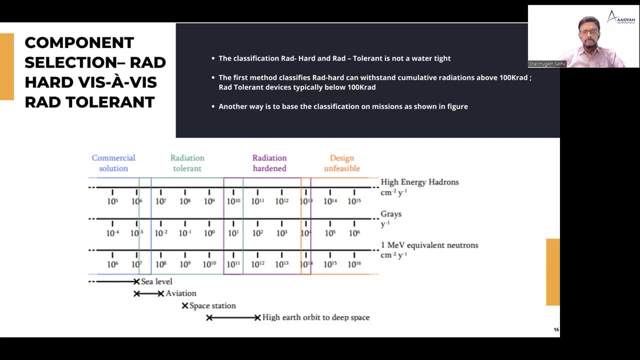 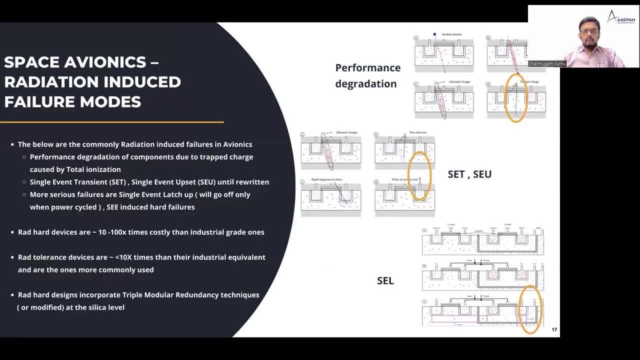 definition can be based on the mission type. Any deep space mission. obviously you need to have equip yourself with a radiation hardened. The deeper you go into space, more the radiation also increases multiple fold. Now comes the. this is the interesting portion of the. 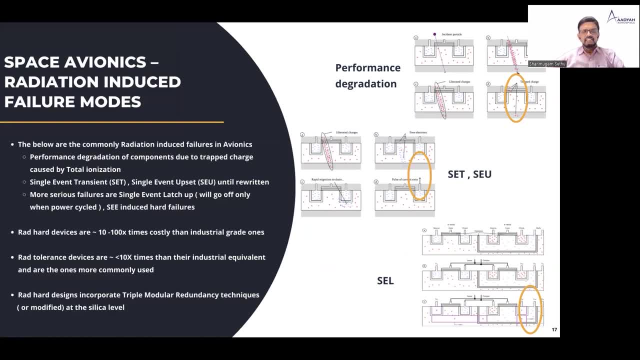 topic today, how radiation is literally able to drive a dagger into your avionics. Now I have depicted here three such scenarios where the radiation can cause a work with your avionics. The first and foremost: on the top. most is the low. 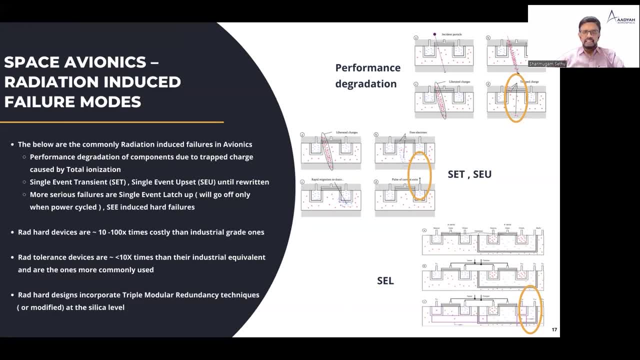 sorry, I'll say low. damaging, That is just a performance degradation. The second, that is just the lack of a reaction. So basically, the reduction of the radiation that you may have in the cell is the reduction of the impact of the radiation over time. 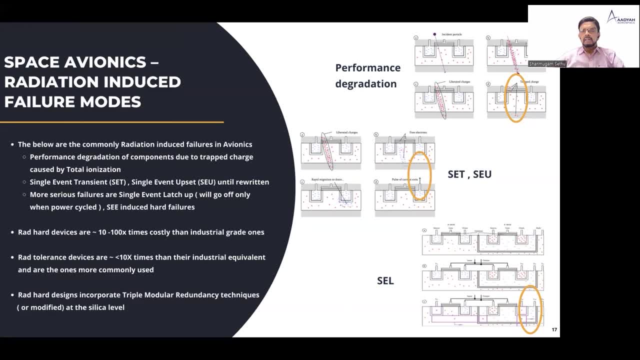 And if your mission is started, maybe able to recover from this radiation impact. What you see on the series of the four charts. there is the radiation coming inside and then you have the additional charge, create charges created within your silica cell And then 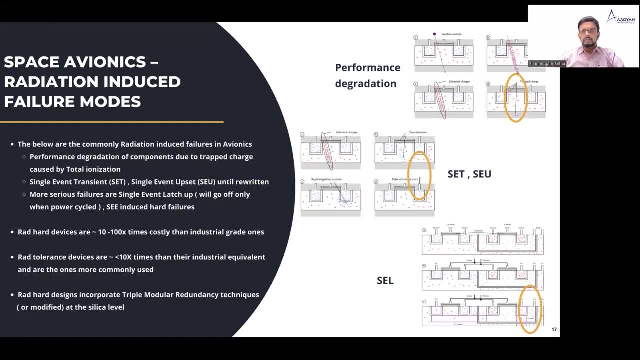 you have the uh, the trapped charges, which are uh present within the silica, and then which degrades the performance of the electronics. so that's the first of the impact you see due to the radiation and the more severe, or in terms of severity, you can put it in the middle. 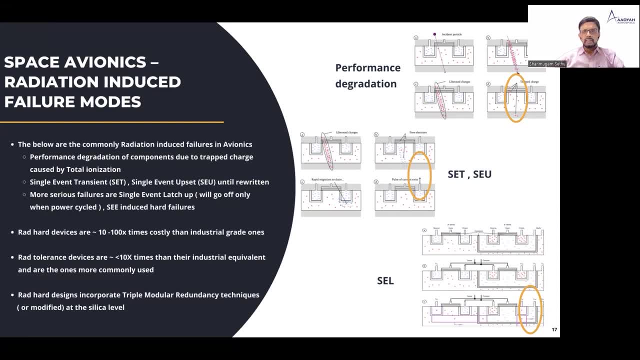 is what you call as a single event transient or the single event upset. so here again, though the incidentary leaves here causes attention phenomena like it can be a current surge going out and then causing an outside electronics to flip its stage, or then it can recover back. 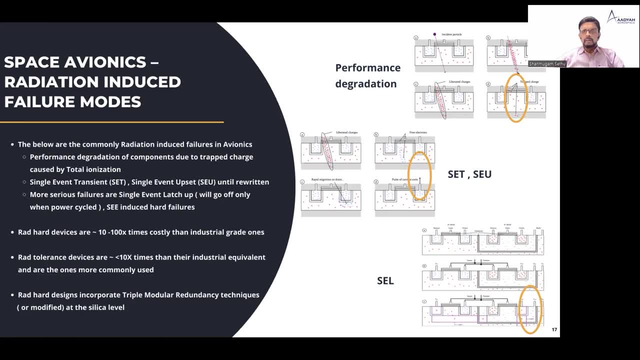 that's appropriately attention type of impact. the other one is that they are memory. memory pitch can flip from a high to low or low to high- that week also, but then it can also come back. so this again we term it as a single event upset for the bottom right. what? 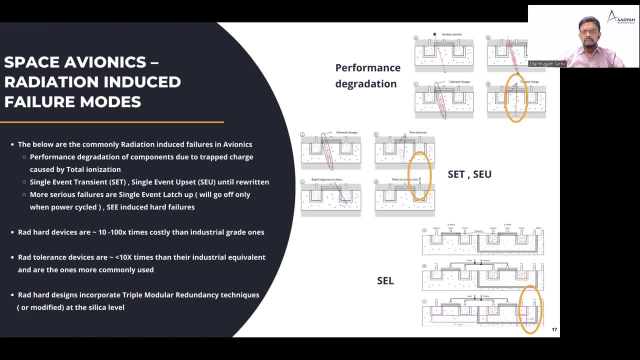 you have is the much, much more damaging, literally, is that it causes the, the radiation causes the latch of these um the memory state or the bit state, and then you can only recover from it by power cycling your avionics, which is again has its own implications. 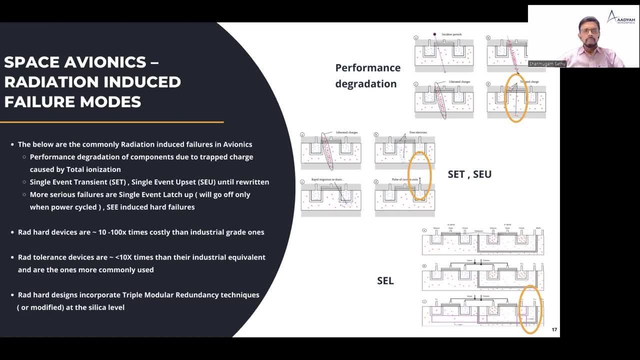 or sometimes it may result in a permanent damage to the avionics. that's what. so this is the. this scenario quite up quite brings out how the avionics can be literally stabbed by the radiation. as such, now comes the consideration between the record. so, in view of all this, we can't go ahead. and then for a rare device, because, for the simple fact, 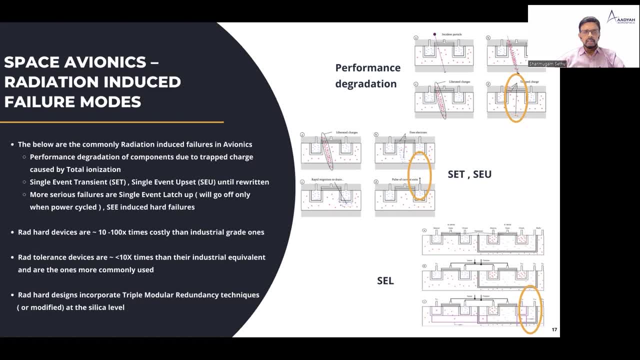 you will blow a hole into the emission budget in terms of the cost, because the cost is nothing, will not be less than 100x times the normal industrial grade processors. the radiation tolerant devices are a little bit gentle on your uh budget. they are around 10x times. 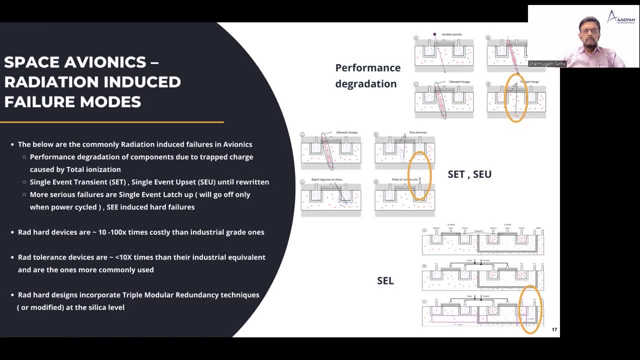 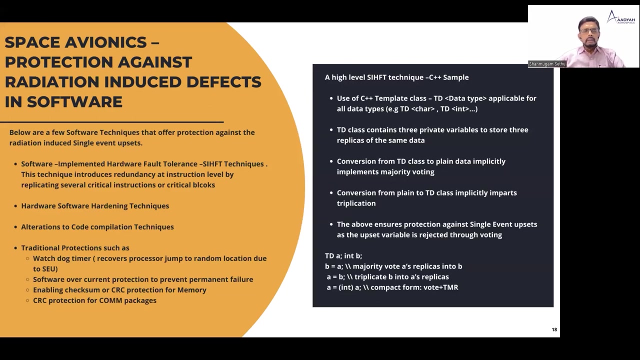 the normal long industrial grade. now here sort of insight why the red hot devices are costly: because the uh, the redundancy to handle the um radiation failures, need to be built into the silica cell itself. with that, let me move on to the uh, the uh. what are the protections we can have? now we know, 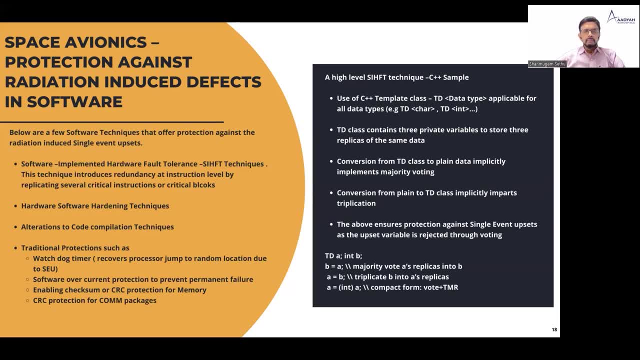 that the we can have to build armor around the device by going for the hardware red hardened device, but there are some sort of a simple techniques which we can adapt. so in this slide you can see that the data software also can play a a very, very uh, intelligent role in guarding you against the radiation induced effect. 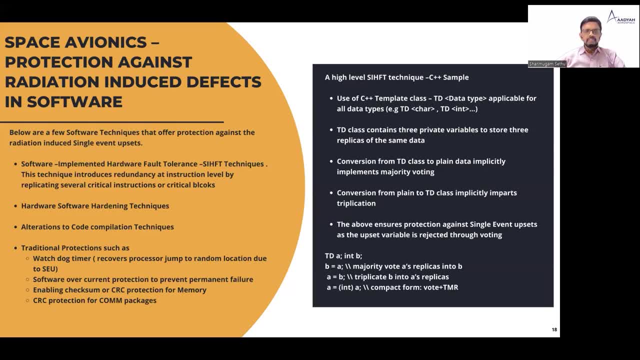 so we have a name for it, called, as the shift of pronouns, a little bit different. or with the i and the h interchange, which stands for the software implemented, hardware fault tolerance. now the for the right, you see a simple programming technique. so from the c plus plus, wherein you can have a very air class defined for your triple redundancy, 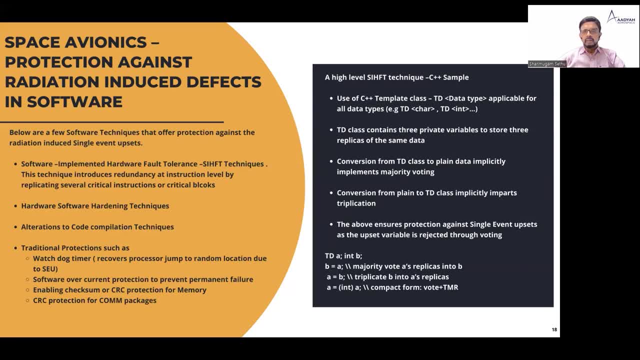 variable and then uh you can buy simple conversion from one class to another, you can bring in the uh majority voting and then you can uh triplication, you can bring it by the conversion the other way around, so and there are other sophisticated way of uh handling the same thing. 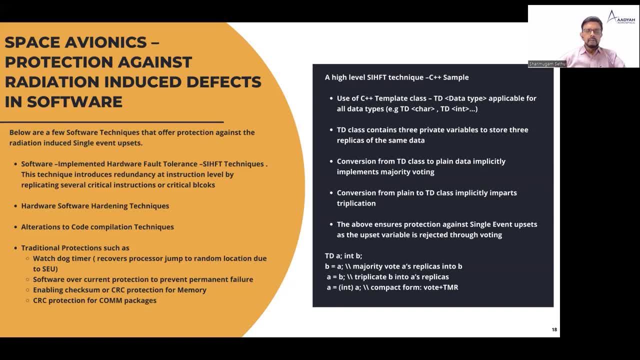 within the software. there is something called as the uh code compensation itself, wherein you can bring in the yeah sort of a protection in software against the radiation induced faults. there are also the uh- traditionally uh- protections, what you built into the software, like the watchdog timer, which are like handling if there is an uh- radiation induced or abnormal, the deduced 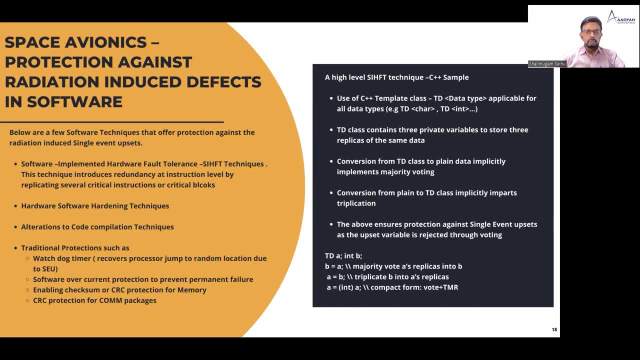 in the operation of the software, the watchdog timer will time out and then reset the browser. there are also, as for the permanent, suppose there is a failure induced and then if there is a monitoring, the software for the workaround that can trigger a protection measure, and then uh, it can uh sort of uh uh avoid the permanent failure happening. it has become. 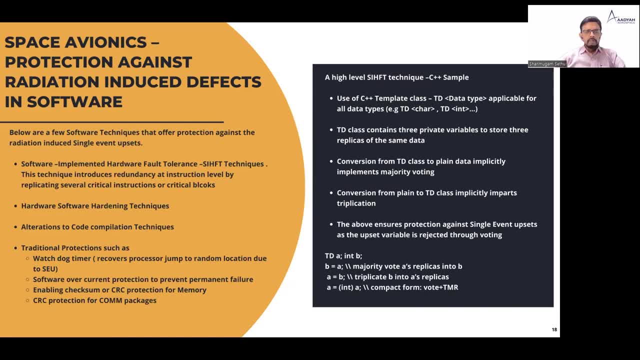 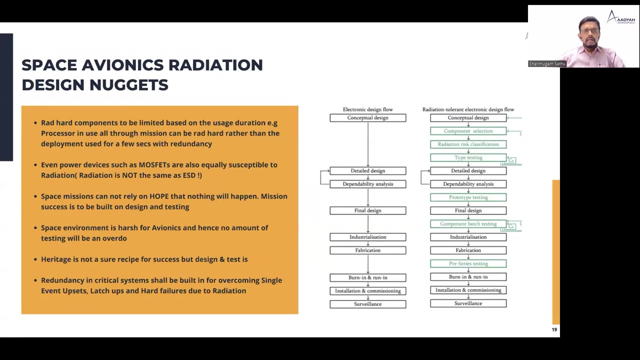 inside the silica. but the other protections is obviously the cyclic tech or the crc, as well as the um for the memory, as well as the communication uh packets. these also will give you a protection against the uh in software, against the radiation effects. now in this slide you can see that uh, even uh. we can't discount anything, uh, any device. 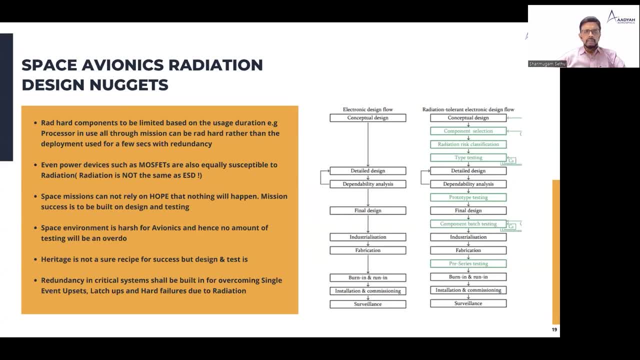 you know electronic device is susceptible in the phase environment for the radiation induced effects. so we can't rely on hope that uh your mission will not have a radiation impact. so it has to be your uh safeguard against radiation failure should happen with another design or the testing also, the uh radiation induced is. uh also means that uh, whatever amount of testing you 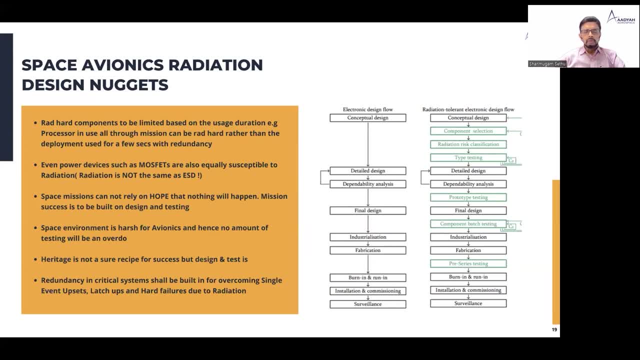 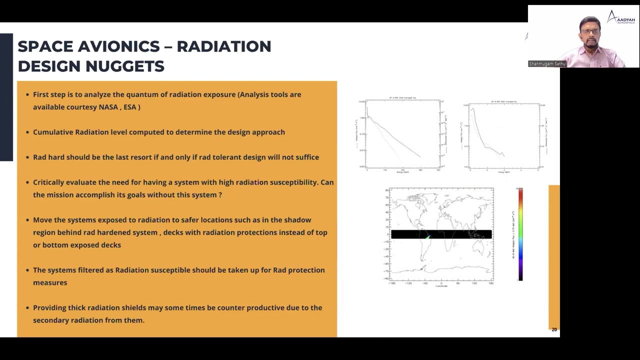 do to simulate the radiation in your outfits. avionic testing will still help you to ensure that mission success. and now the uh other thing is that uh redundancy of the critical system is one more step, so it should essentially take it to overcome the radiation induced effects. now, with respect to the radiation, what are the design nuggets? 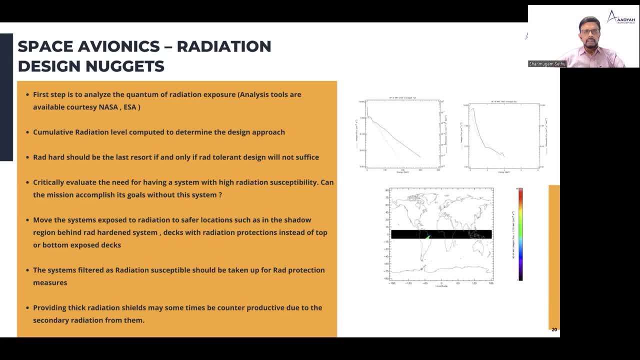 or how do, what is the best practices which which you can adapt so that we make our avionics or radiation uh defect proof? first and foremost is that you need to evaluate what is the quantity of exposure uh your mission will encounter. thankfully, there are enough tools available. 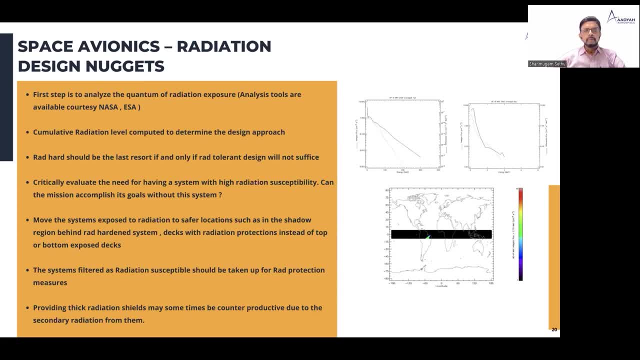 courtesy nasa or etsc by which you can do your analysis. whatever graphics you see on the right hand side is one of the analysis done at uh, at the uh for a satellite mission and uh you can uh depending on the, the total uh ionic dose or tit, what uh you have this analysis, uh throws at you. you can decide whether. 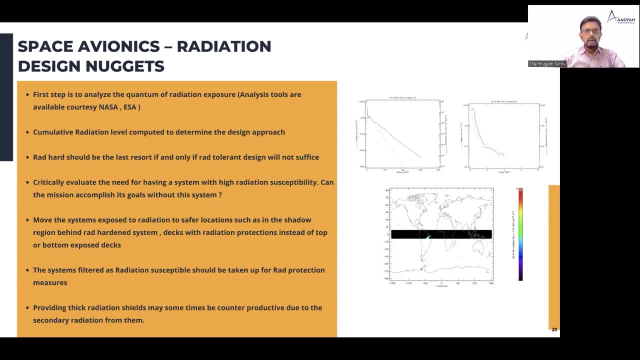 you need to go in for a radiation-hardened component now. don't jump in into the radiation audit component because of the cost. we can also uh. i really think your design architecture whether you can do away with a system which is uh radiation has a high radiation capability. can you substitute it with the? 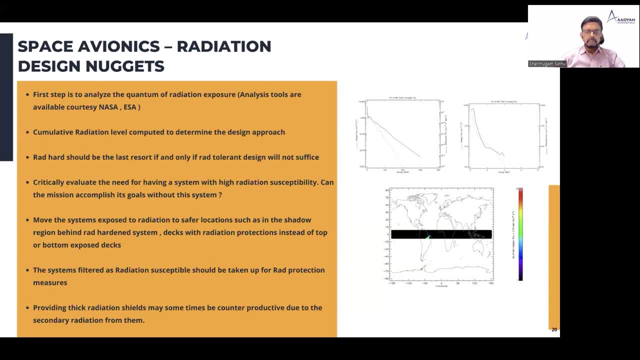 their generic system, which is already the additional, can implement the functionality within that radiation northern system. an example will uh probably make this what uh this um step very clear is that suppose you are uh having a navigation where dedicated processor- this is like uh usually the lunar landing- there is always a dedicated processor because of the uh. 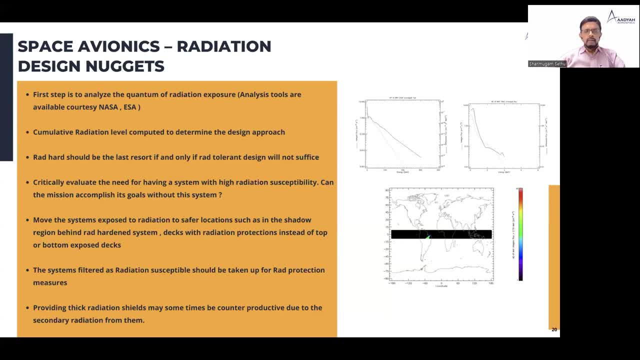 processing speed requirements Now that higher processing for the landing, whether it can be combined into a radiation-hardened main onboard computer instead of having a separate eatable which the processor the landing navigation process. So these types of decisions you need to essentially go through because of the higher cost of the radiation-hardened components. 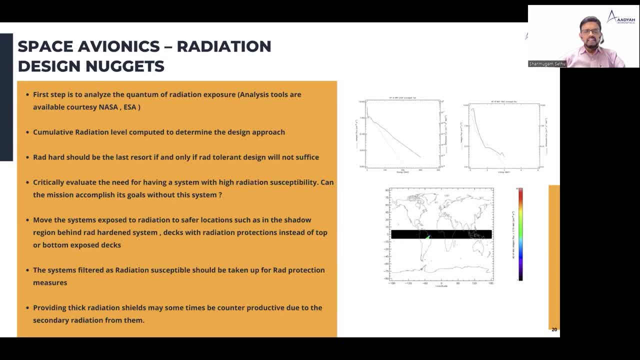 There are also some of the tricks which are very simple. Again, you can move the radiation-suddable system into the shadow of the radiation-hardened system, can simply hide it or tuck it away inside your spacecraft in a place where the radiation is. 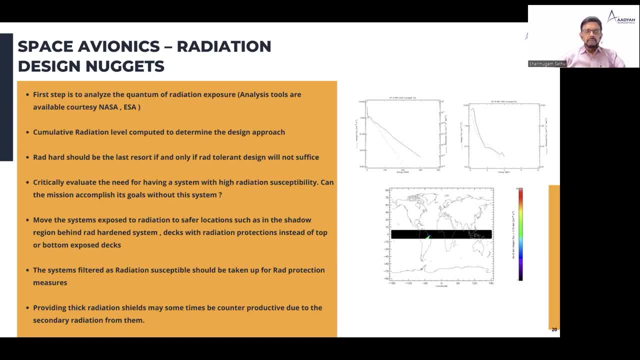 expected to be minimal and we have some protections which are covering up like, for example, you can always move your radiation sensitive system into the middle deck if you have some top deck, middle deck or the lower deck of your spacecraft. so the the other thing is that the normal. 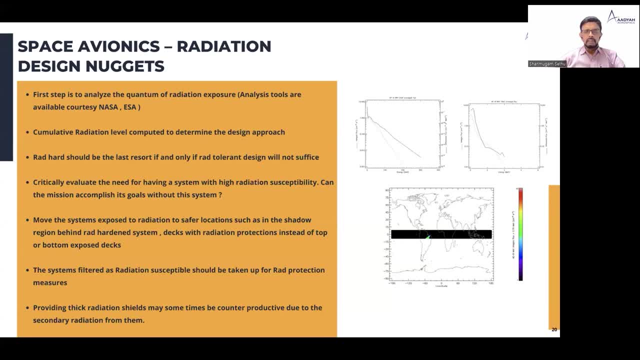 action taken. whenever you see radiation susceptibility and then your probability of the higher total ionization dose, you tend to put in the higher or a thick radiation sheet. but there is a danger in that one. also some of the materials to use for the radiation shield or prone for air phenomena called as the secondary radiation. 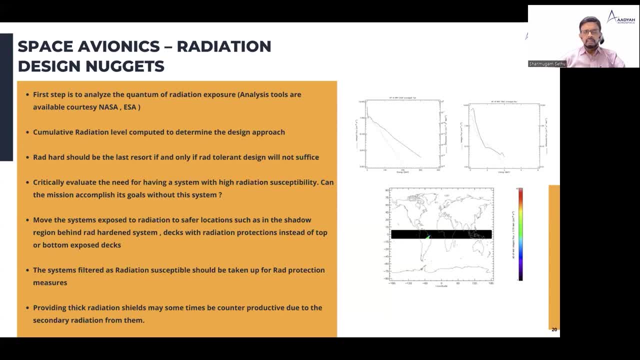 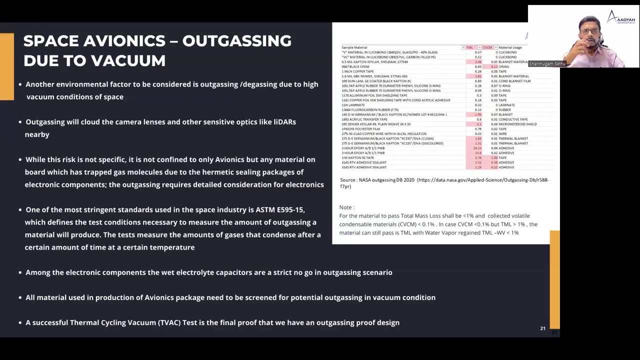 so providing just a thick radiation shield is not a 100% pull through against the radiation, because that same thick shield may give rise to a secondary radiation directly hitting your shielded avionics. okay, i think we have got enough of the radiation, let's go to the next slide. 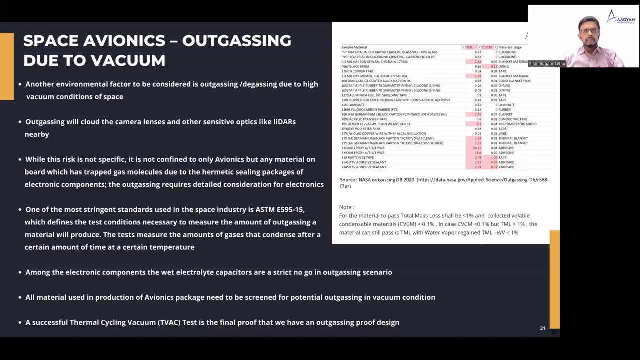 okay, i think we have got enough of the radiation. let's go to the next slide, moving to the other uniqueness of the phase, avionic, which is caused by the vacuum environment. we call it, in terms, outgassing. this is because of the vacuum conditions. so all the trapped gas, gaseous molecules or the 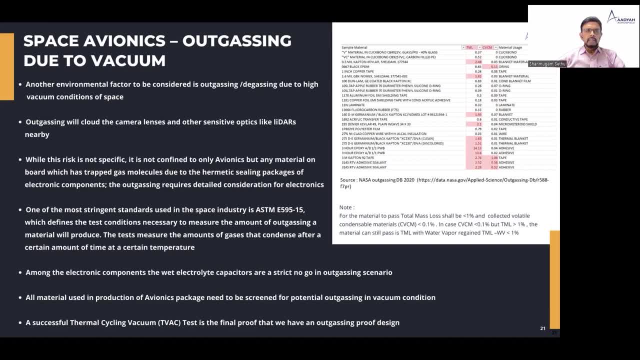 particle is, will tend to outgas from any device there, let it be a plastic or a glue used or a grommet used, or it can be, and, or it can be an avionics package having a tractor of gaseous molecules, or it can be a connector. it can be. so, the moment the avionic goes into your vacuum, this 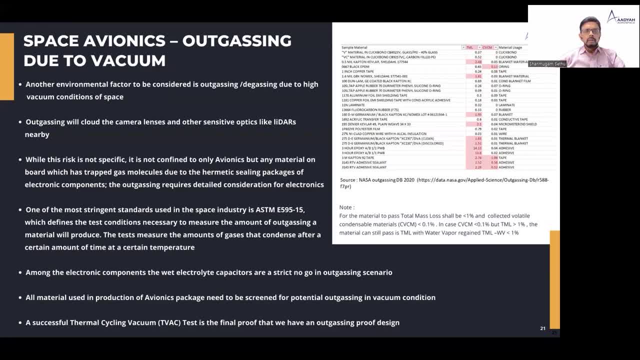 outgassing automatically happens. now it is not that this gases can passively escape into the phase one of the natural law after. our effect of this outgassing is that you will get your sensitive optical components, such as the camera lenses, will be clouded by this, and sometimes it can be as 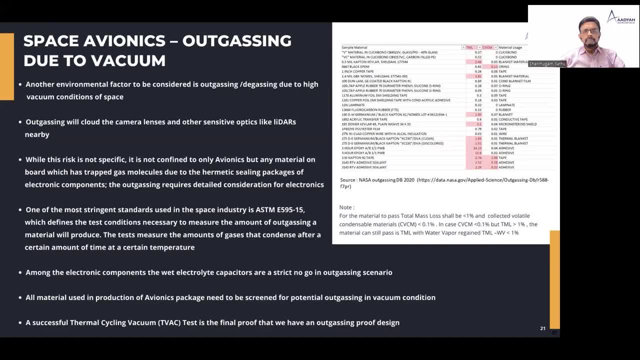 severe as some of your- the laser lidars which you use for the navigation, the crater navigation on lunar landing- those ones also will be clouded by this. and sometimes it can be as severe as some of your the laser lidars which you use for the navigation, the crater navigation on lunar landing. those ones also will be clouded by. 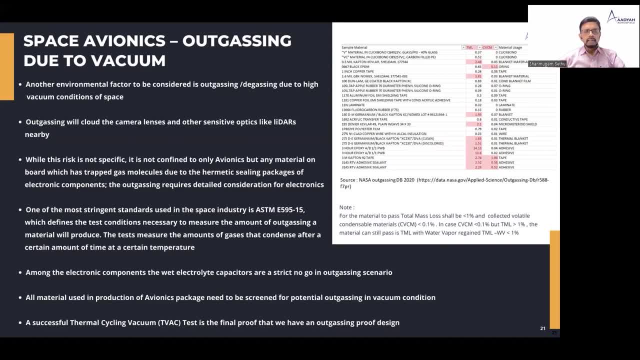 your outgassing outgasses and then they become or degrading the performance. so the one of the ways is that, um, you need to look for what is the uh component which is usually in the avionics, which is prone to the outgassing risk, and then you need to test it out. 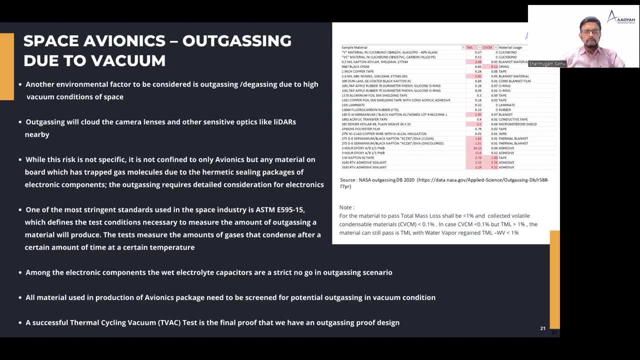 and uh, in spacecraft mission, nothing is left to us down. there is a the entire spacecraft may go to what you call as the vacuum test, or more precisely what you call as the t-vac or the thermal cycling combined with vacuum. and uh, it is not uncommon to see uh entire fair spacecraft being uh subject to. 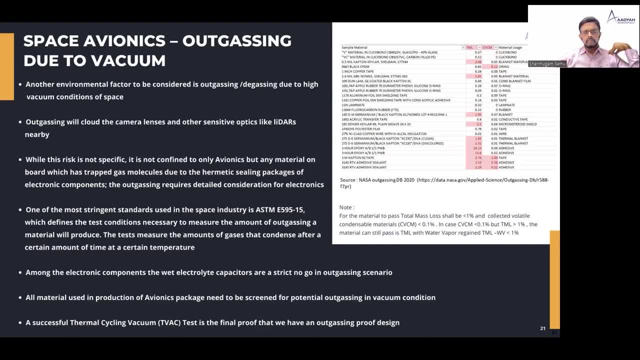 this vacuum and the way the test is being just judged for uh, their pass or a failed criteria is very simple: how much is the reduction in the mass due to the uh outgassing and uh, how much is the uh, the, the quantum of the gas which is the? 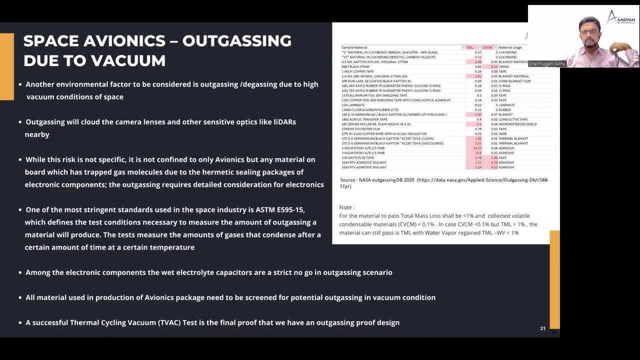 come out of the sample at the test. so these two parameters determine the total mass loss should be less than 10 percent, whereas the uh, the condensed uh, volatile condensable material, cdcm should be less than 0.1 percent. unless we meet these two criteria, we can't completely say. 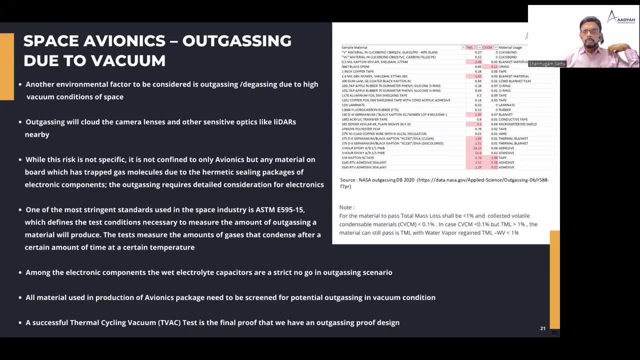 that even after the very first test with this uh sample. so i think we have a very nice uh, uh outgassing proof of uh safety and i don't see that we we have a full proof for uh outgassing proof for avionic design, the some of these uh obvious uh. 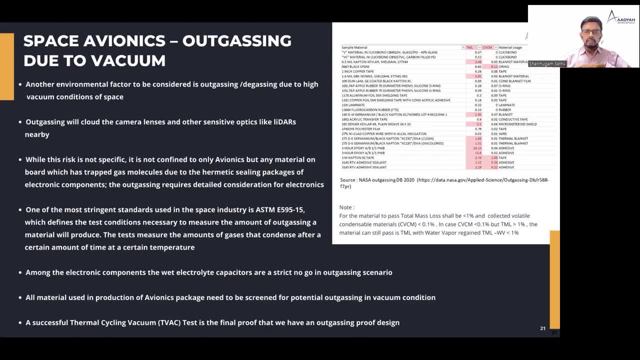 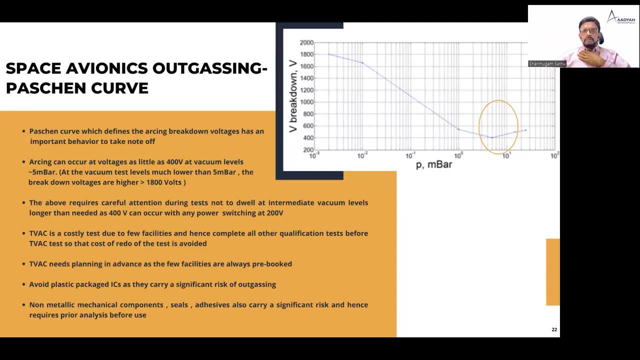 spoilers for your avionic design. in backbone will be the um to vet the electrolytic capacitance. so it's a strict uh no-go. as far as the phase avionic is concerned. which I want to touch up is that don't think that your risk just goes up with respect to the vacuum. 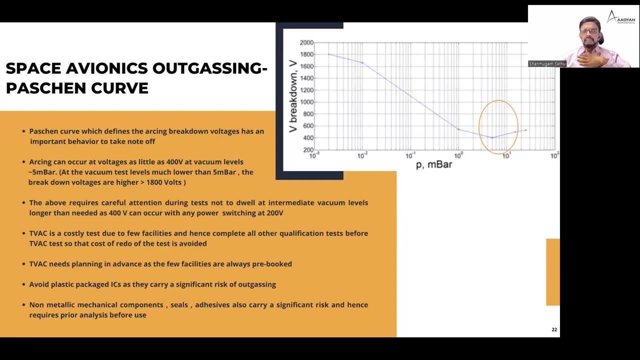 level, There is a phenomenon which is characterized by what we call a Sebastian curve, and that is a curve which has the vacuum plotted against the breakdown voltages and, strangely, you have a possibility of a breakdown or the arcing in case of a vacuum condition happening at. 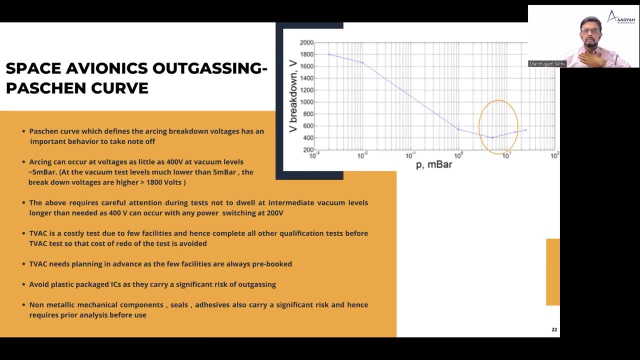 a voltage as less as 400 volts at around 5 millivolts. So this means that not the higher vacuum levels is going to cause you. however, it also something as low as 500 volts. So this means that not the higher vacuum levels is going to cause you. however, it also something as low as 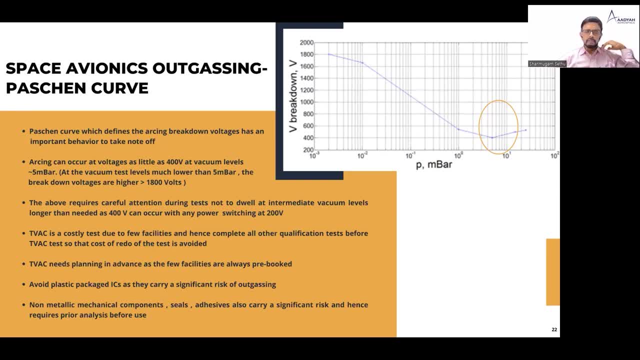 around 5 millivolts Also poses a risk to the avionics, especially if you consider the tracks. I just entered the PCB as such. So suppose you have a MOSFET bridge and then you have the two tracks running a MOSFET bridge, operating at around, say, 115 volts, may have a spike of around 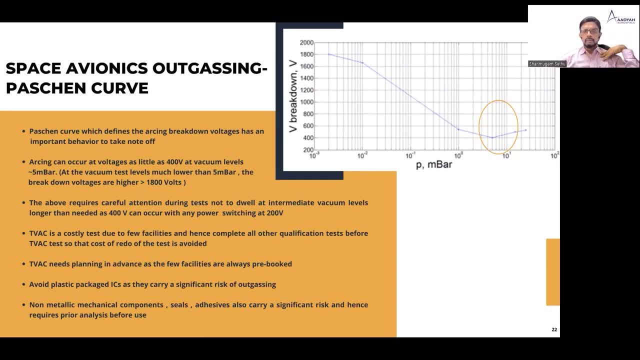 two to three times and the transients, especially during the switching of the MOSFET, and that can easily cross the limit of the voltage and you may have a spark over between the two adjacent tracks if it crosses around the voltage. So that's again another consideration. you need to make it while you design your. 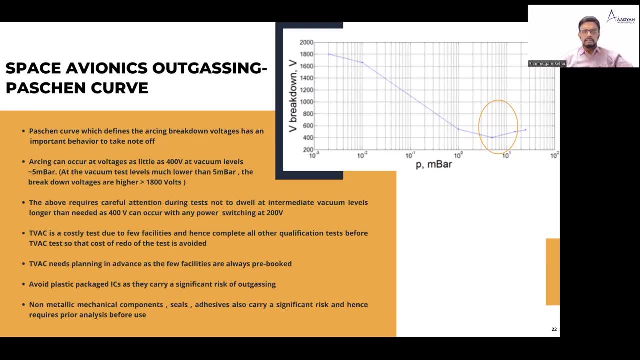 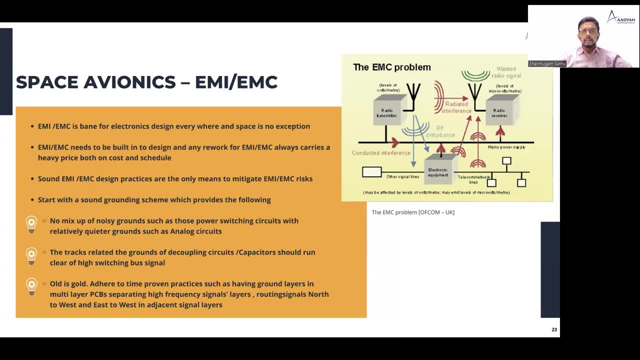 PCB layout which are subjected to higher voltage transients. Now comes the traditional risk of any avionics system, whether be it on ground or be it on space: EMI-EMC. Let me quickly jump in, because anybody who is dealing with avionics, for them, EMI-EMC will be a 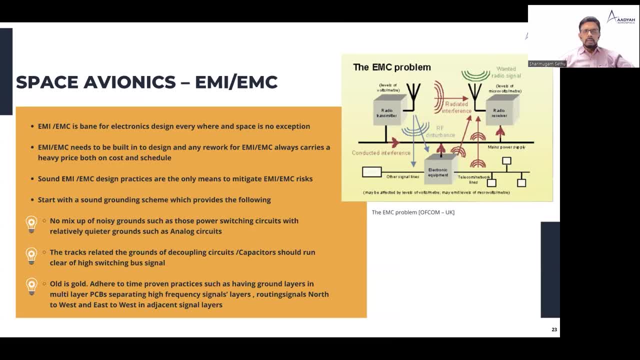 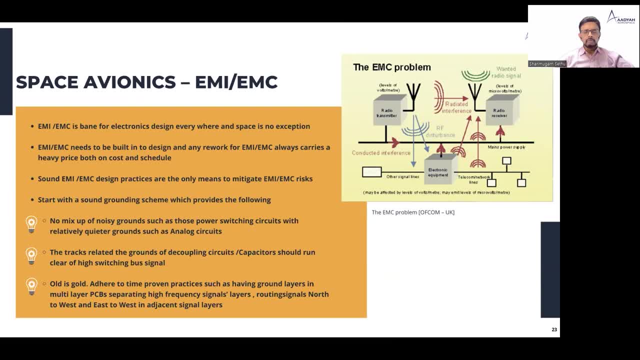 you were switching right from your pc layout to your layout or the entire avionics, and especially the routing of cables or routing of the tracks, and you also need to pressure care about the decoupling circuits and also your grounding ski. So sticking to the basics of addressing the EMI. 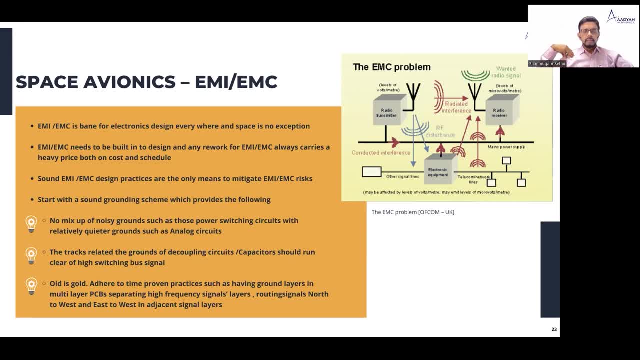 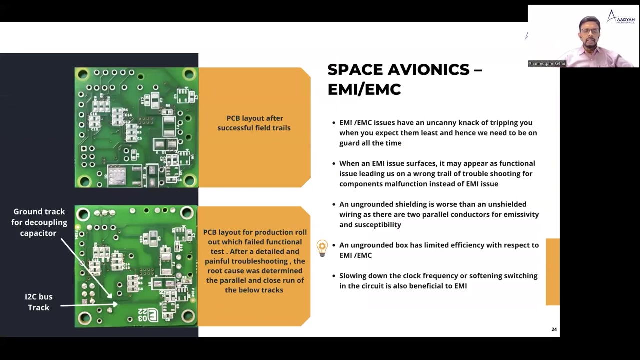 EMC may still be, can help you with respect to the phase avionics. There's nothing different which you need to take as far as the phase avionics are concerned, but you need to stick to the basics. Just an example of how we can see our little bit of oversight cancels out with respect to EMI. 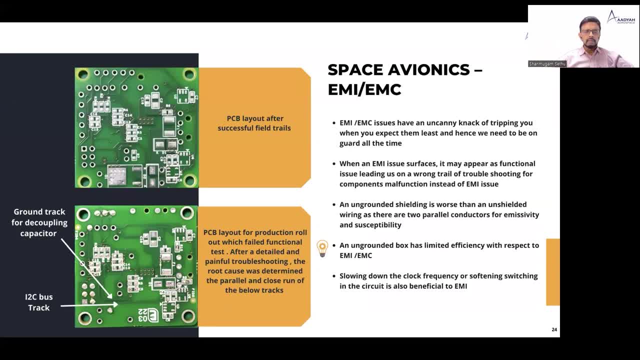 EMC or the bottom PCB. You can see there are two tracks which are hardly more than 10 mm long. One of them happens to be a decoupling capacitors ground track. other one is I2C bus track. Now, just this less than 10 mm parallel run. 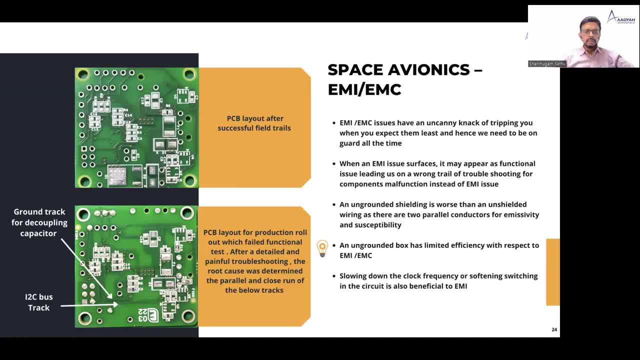 is sufficient for the noise coupling due to EMI to disrupt the operation of the I2C bus track and then the entire board would not be operating. Just to illustrate the care we need to take with respect to the speed out Also, keep in mind, I mean, if you just connect all your grounds to your 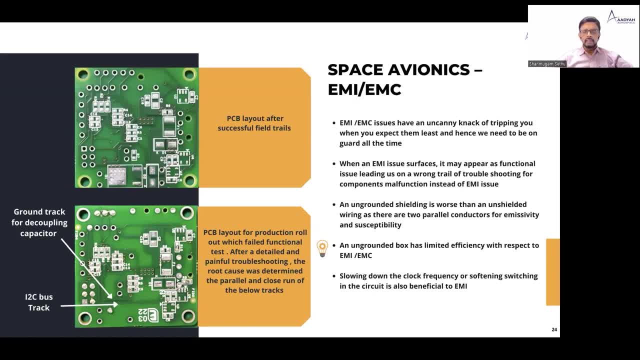 box chassis and then the chassis is still floating in the space. you don't have a sort of a luxury of a metallic structure combining everything, because the facecraft is a amalgamation of different components and it is not a metallic structure completely imposing. so your grounding efficiency may not be right, and if you 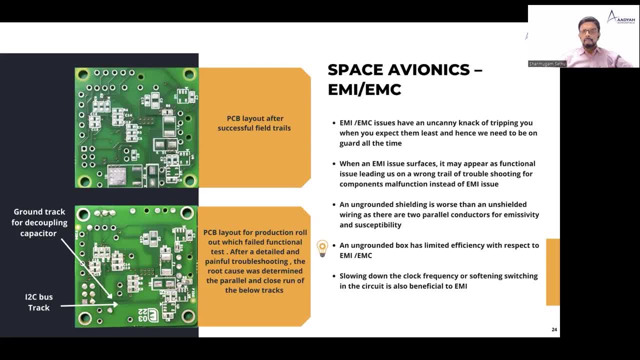 end up in an ungrounded box of avionics is as good as uh not having a yeah emi emc protection apart, because, uh, your entire ema emc protection is built upon having an efficient uh path for connecting out your nice currents. you can also adapt the uh the methodology that tricks up to 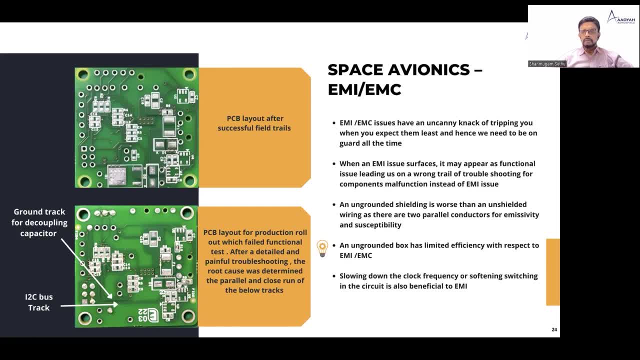 the design of the avionics, like you can slow down the clock frequency or you can make the transitions a little bit slower with respect to rise time or the fall time. that will also give you much dividend with respect to controlling the mi amc on your circuits. 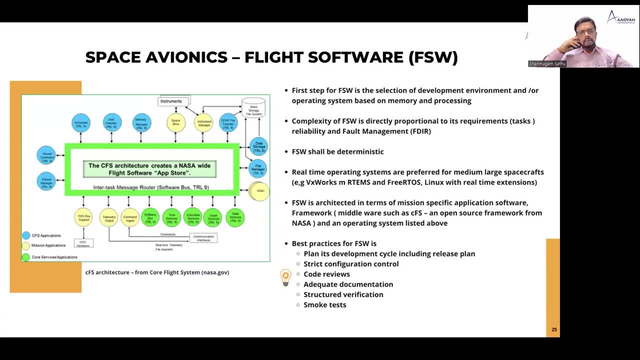 now i'll let me cover the uh sort of uh, give you an insight into the how the flight software or the software running on the phase avionics look like the uh the normally you have uh on a larger spacecraft. you have operating system, you have a middleware. 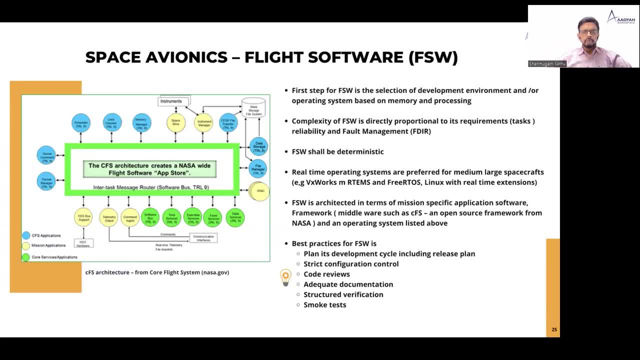 which is uh, there are enough open source available from the nasa. uh, like the core flight system is one of the commonly used middleware, then you build your application on top of it and the best practices with the flight software is no different from what you do on the safety. 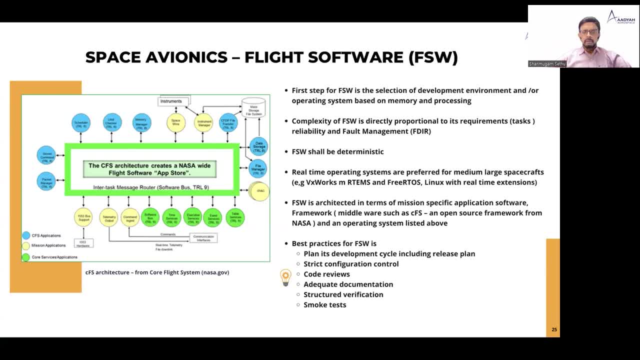 critical software on ground. you need to plan your development cycle with the sufficient checks and balances. you need to have a strict configuration controls. you need to do your code reviews. documentation is the key for us to uh have ensured that the software is uh made as per the requirements and uh it's verified as per the comments. and you also have to have a 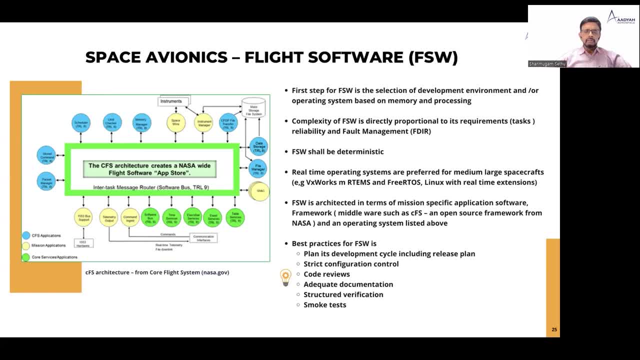 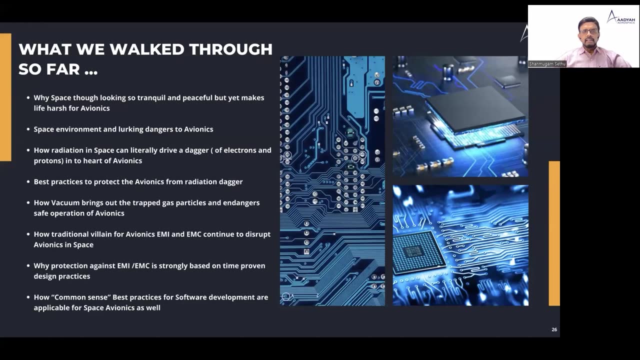 robust verification and the smoke test as the software evolves is also a good way to ensure that your final software it doesn't have any major bugs. okay, let me. let me summarize, uh, what i have, what we have been talking this evening. we have the uh, first and foremost we looked at. 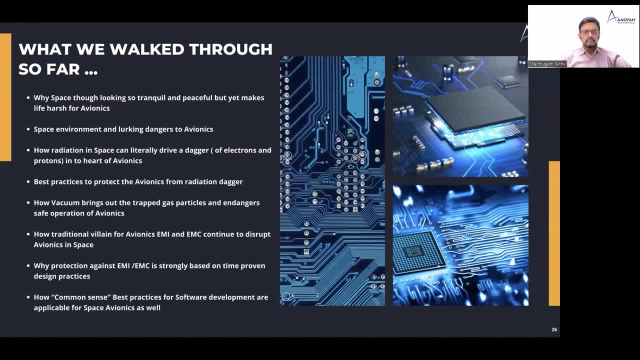 why the space is harsh as far as avionics is concerned and what are the dangers which are hidden in the space for the avionics. we also consider how the radiation can literally drive a dagger into the avionics. we also consider- we also talked- 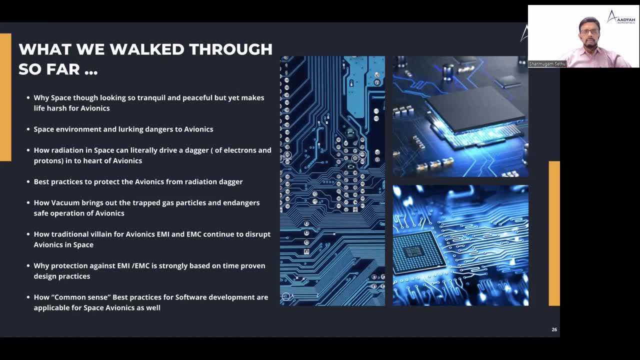 about what are the best practices to prevent such a damage to the avionics due to the radiation. we also talked about what are the impact the vacuum brings on the avionics. we also talked about the emi fcsh for the phase avionics procedure. 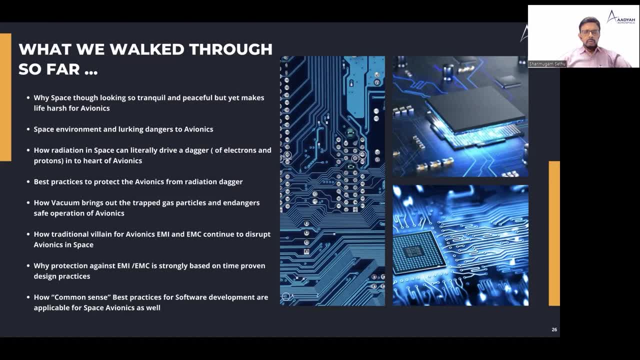 what are the best practices to prevent such a damage due to the radiation. we also talked about what are the best practices to prevent such a damage due to the emi fcsh for the phase. so the other. what i want to leave you with a thought is that, uh, except for radiation and 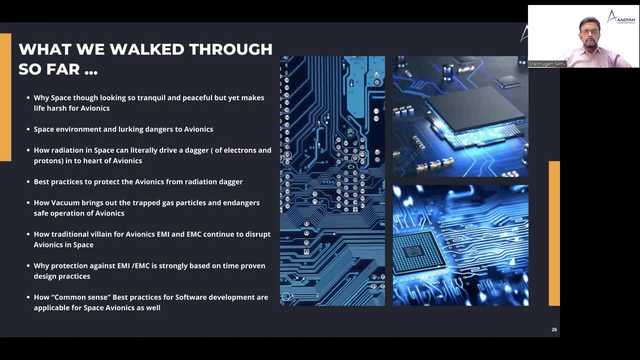 gassing. the other practices with respect to emi, emc or the. the software is uh. again, we need to depend upon the best practices we follow for their ground-based software. we need to take the official precautions with respect to radiation at the vacuum. So with that I will hand it back to Abhirami. 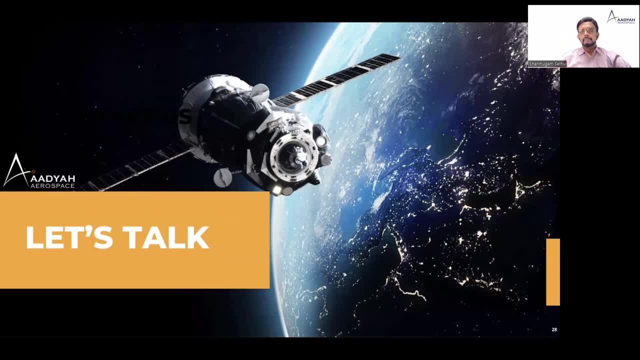 Thanks everyone. Thank you, Mr Sethu. I'm sure that was quite an insightful session for our audience. Now we move on to the Q&A. Please feel free to drop your questions in our Q&A box. We have a few already in here. 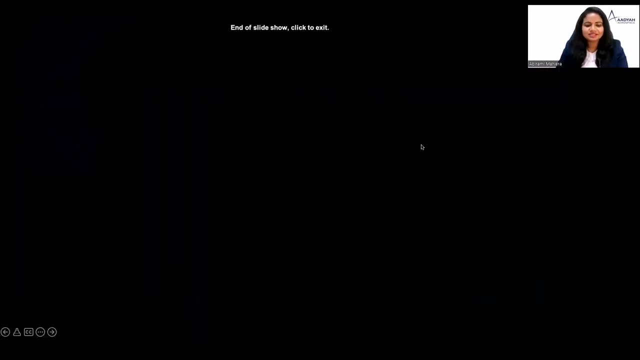 Let me start with the one from Mr Anish. So what he asks is: if the temperature difference is substantially large between the sun side and the dark side on a satellite, can thermoelectric generators be used for generating power within the thermal management systems? 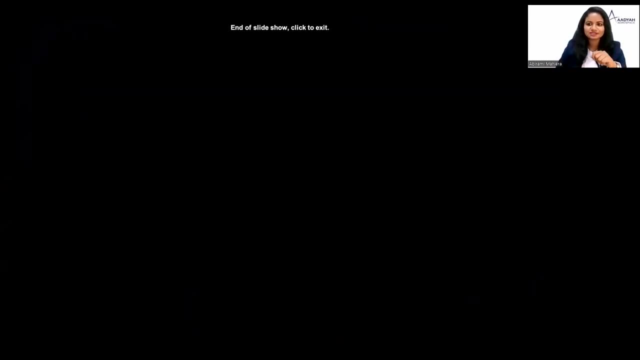 So, Anish, we are unmuting you so that you can have a direct interaction with him. Please introduce yourself And please go ahead. Hello, Yes, yes, Anish, Yeah, I'm Anish. Yes, Yeah, very interesting session. 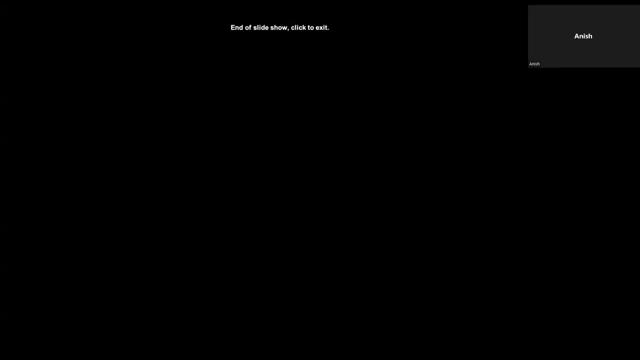 Got to learn a lot about space avionics. So, yeah, I had done a project back in college where we used thermoelectric generators, So I just wanted to know if the heat difference between the dark side and the sun side is so large. 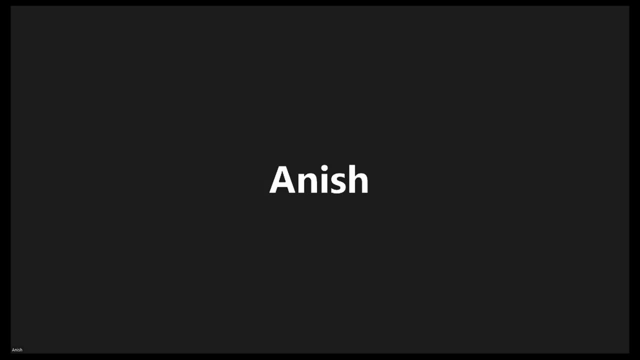 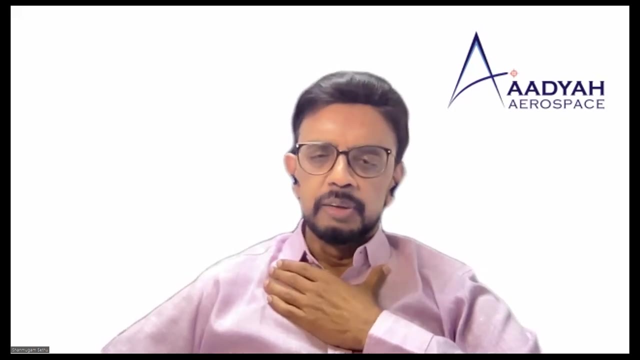 why can't it be used on space satellites? And what's the difference between the dark side and the sun side? Yeah, I mean there are some thermoelectric generators- we call it that. So there are some of them, ones that have been used, but not as a primary power source. 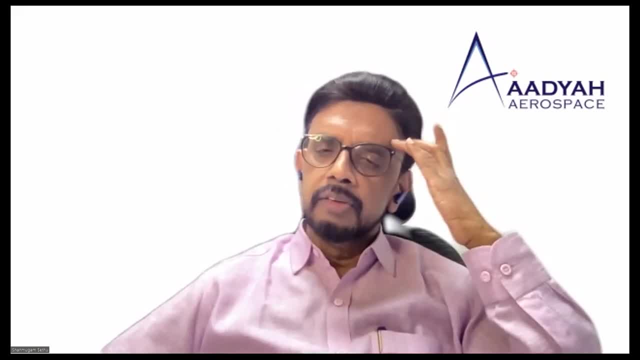 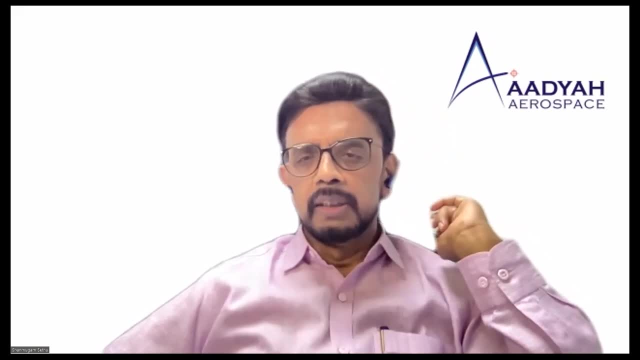 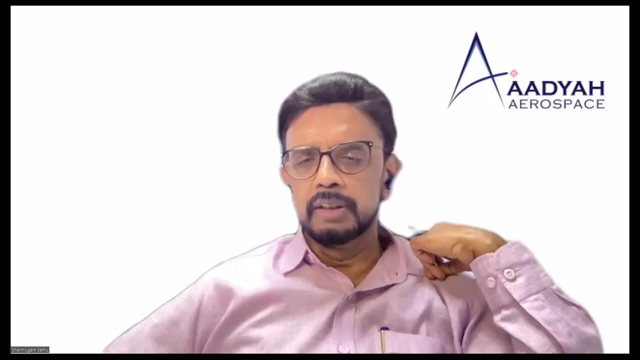 But because the other than the solar, the only other primary source that has been used in the space missions is the radioactive thermoelectric generators, So RTGs we call it. The thermoelectric effect has been experimented and then, but not a very, very stable usage with respect to space missions. 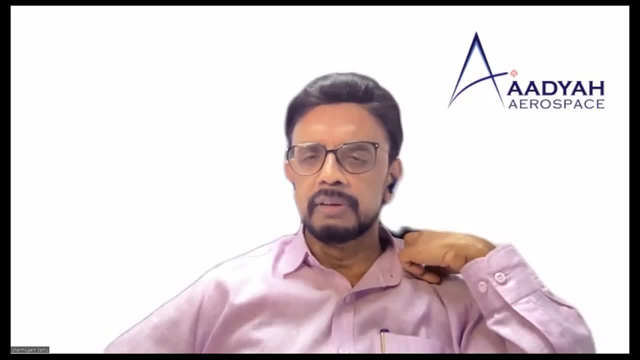 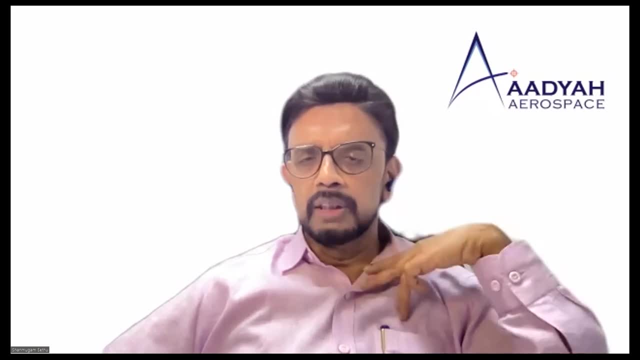 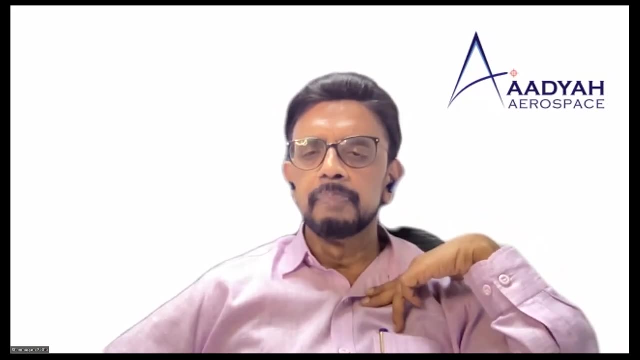 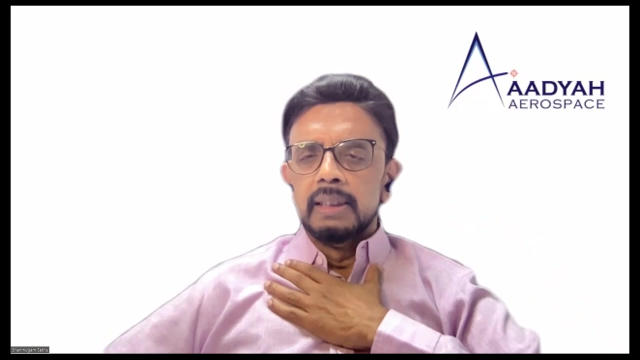 I do agree with you that the difference in temperature is large, but again tapping it and then building an efficient thermoelectric generator and not blowing your mask, But most of the things, what you find are even the other raw energy sources, Like, for example, the fuel cell or any other source which you did. they are all very attractive as far as the conservation of our alternative source of the power. 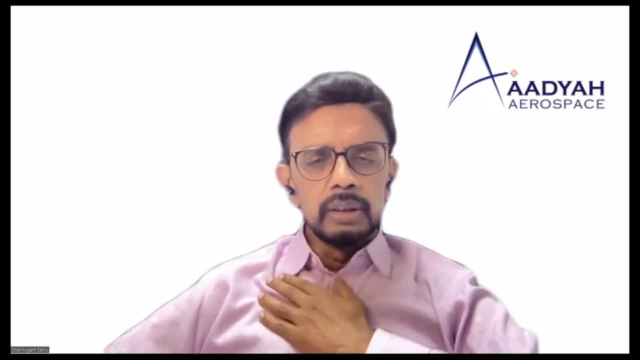 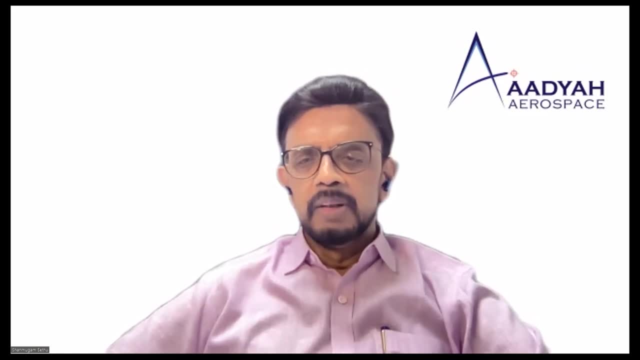 But what finally decides whether they are going to be used in a space mission is: how are we going to meet the mass budget? So it is a tradeoff between the mass of your alternative power source system. Again, it's the conventional one, Yeah. 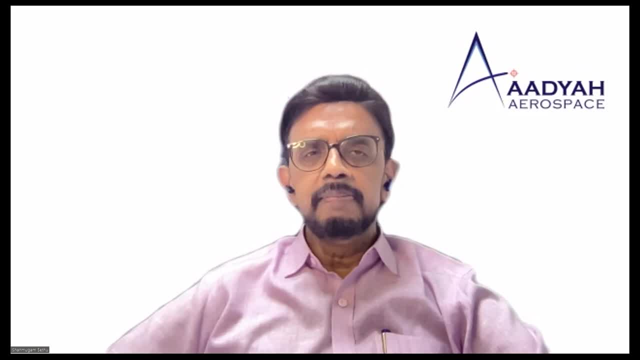 Yeah, So thank you so much for answering my question. I just had another quick question. Like you mentioned, the shielding radiation from shielding the satellite from the radiation. I've also heard that Kevlar is quite effective in blocking out the radiation. 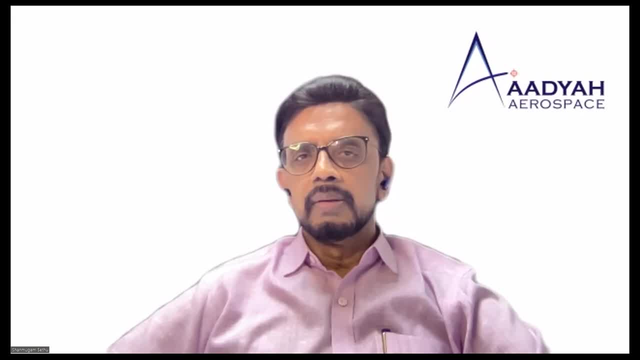 Is it still used or has it been used before? Come again, Nanish. I didn't hear you properly. Yeah, I just wanted to know if Kevlar is being used to protect satellites against the space radiation. Oh yes, I think all the radiation sealed materials have been used and there are new materials also been researched upon. 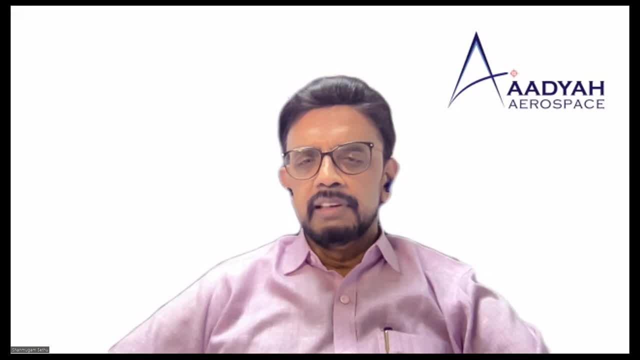 As I was mentioning during my topics, the main criteria is that are you going to have an optimum mass for the shield which you are putting And are you free from the secondary radiation aspect? So there is a whole gamut of the shielding which has been used, but the key consideration for selecting your shielding material will be the mass, as well as how effective they are with respect to providing the shield. 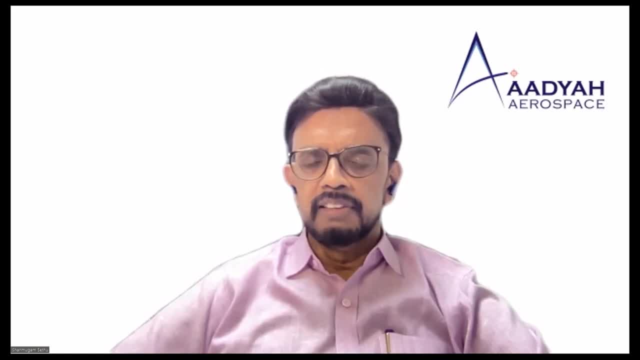 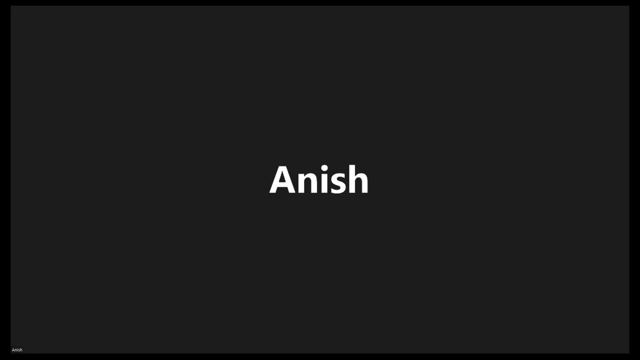 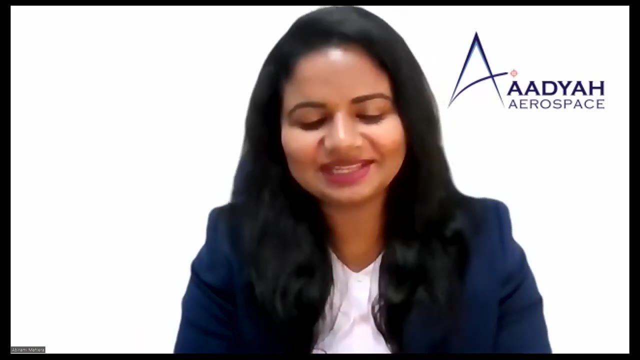 Yeah, Yeah, Yeah, Yeah, Yeah, Yeah. Well, thank you again for answering my questions. I think that has cleared all my doubts, Thank you. Thank you, Anish. Yes, That was great. I hope that helped you so well. 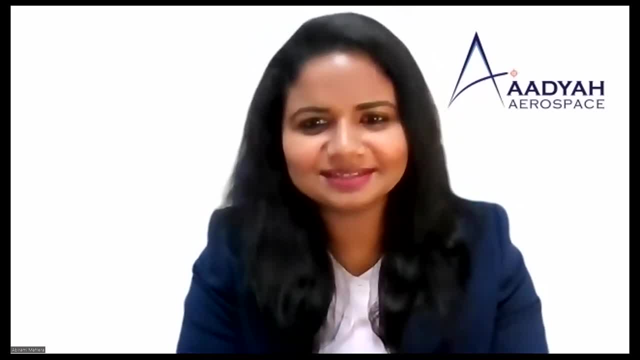 Okay, So we have another question, which is from an anonymous attendee, actually. So what the person asks is: in your experience, what factor is most overlooked in the development of avionics systems? that comes up in the testing phase, Okay. 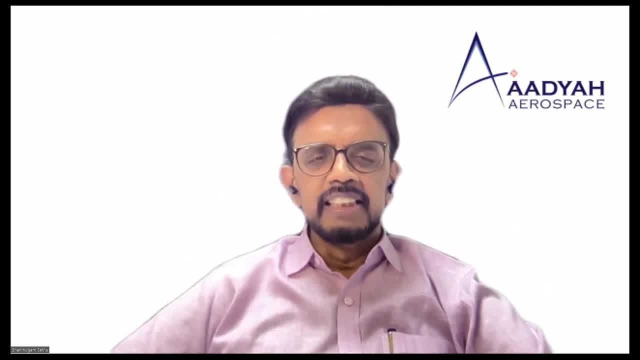 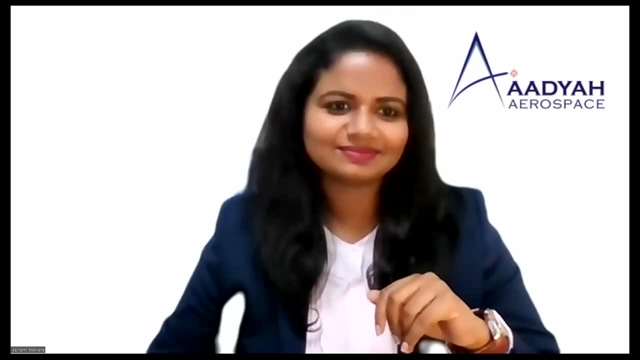 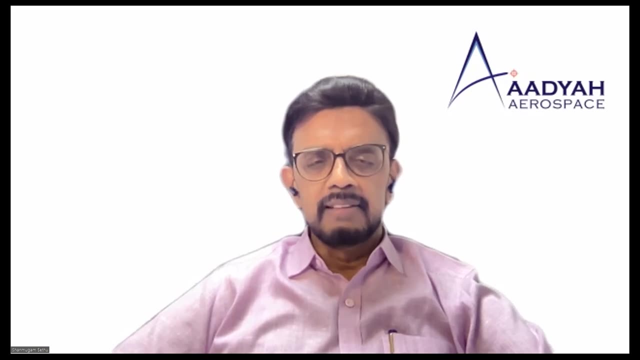 And that is one more Interesting question. Thanks for it. And there are two things. One is that the outgassing is something which tend to be always overlooked And then, once you end up during your thermal test, once you are having an outgassing phenomenon noticed. that is something which is unique to the phase avionics. 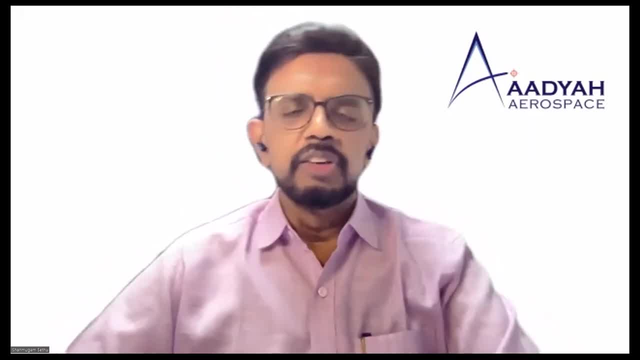 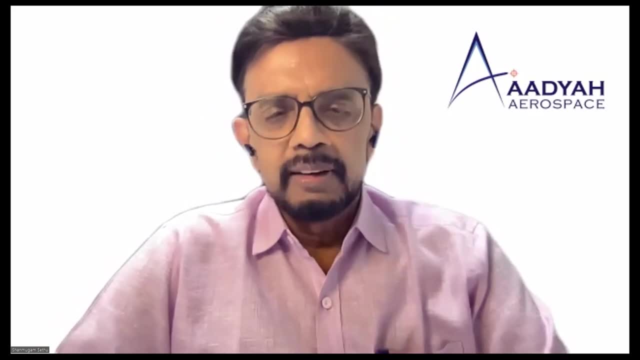 And not many designers tend to look at it. It is just because the outgassing phenomena is so complex. Sometimes it may be the ingredients which goes into making a component, So that is something which I feel is most overlooked. as far as the development of the phase avionics, 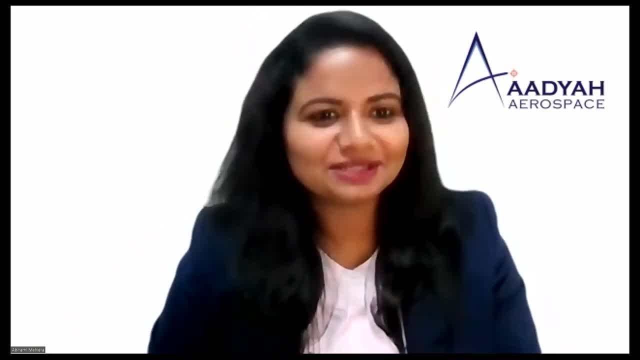 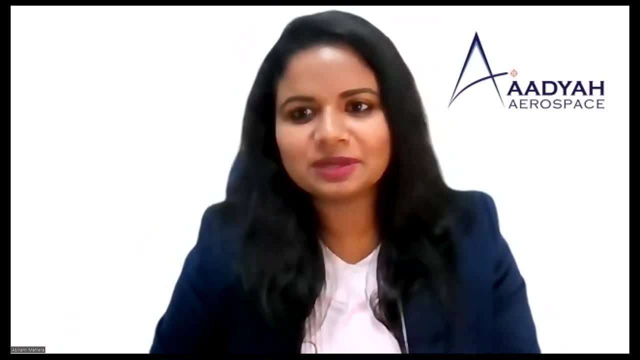 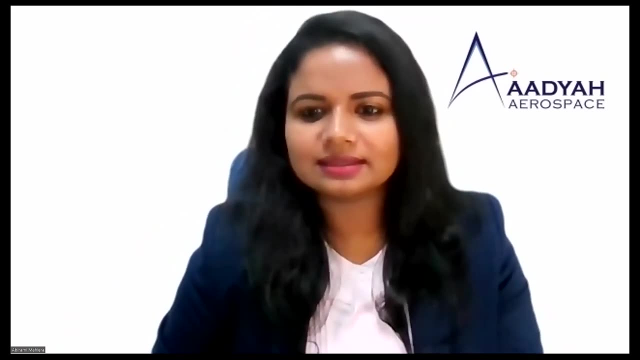 Oh, I'm sorry, I was on mute, All right, So I hope that helped. So we have another question from Mr Shubham: What kind of processor you will suggest for space-based solar power satellite based on microwave technology? I think Shubham left. 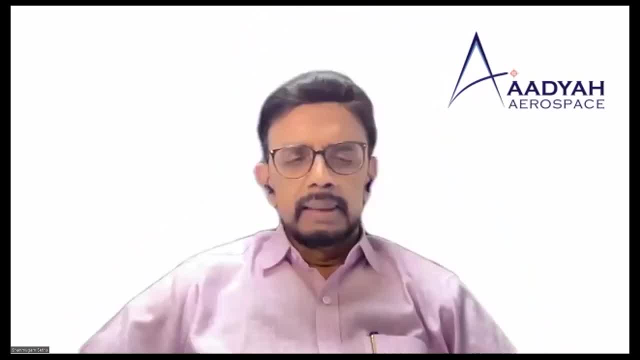 Okay, Okay, Yeah, Please, Shubham. Yeah, I think the process selection is very, very important. I think the process selection is very, very important. Okay, Yeah, I think the process selection is very, very important. 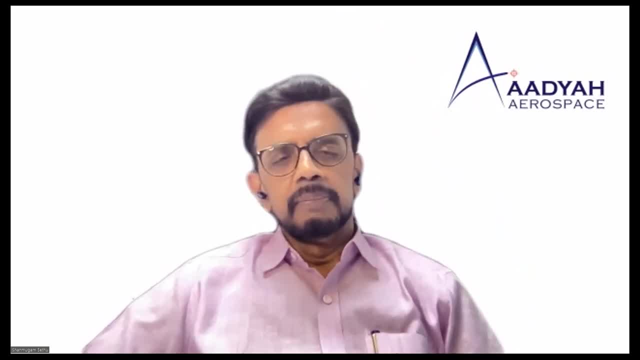 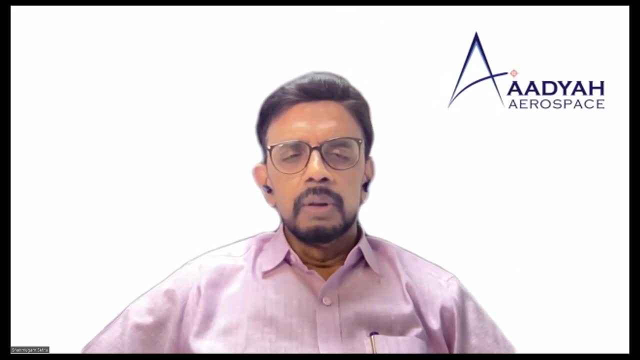 I'd say the exercise, which needs to be carefully done. I will not suggest anything But, as you find in the deck, the most of the process selections, whether you're going for cards or any other custom design or the specific process that depends upon the size of your 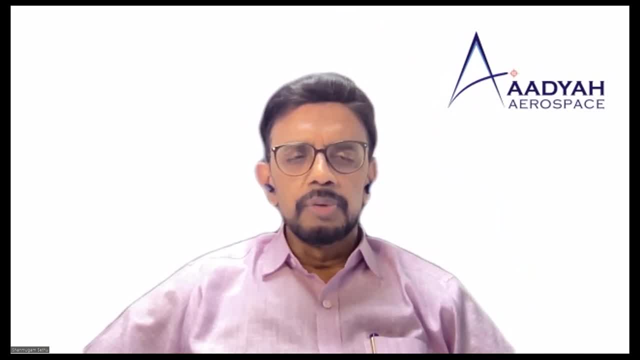 spacecraft. for example, for a CubeSat, there is- at least to my knowledge, there are- around nearly a hundred type of proven flight proven cards processor solutions available. so it's a question of matching your uh, the available processor, to your mission requirements. so the straight answer will be that, depending on the size of the mission and the task which 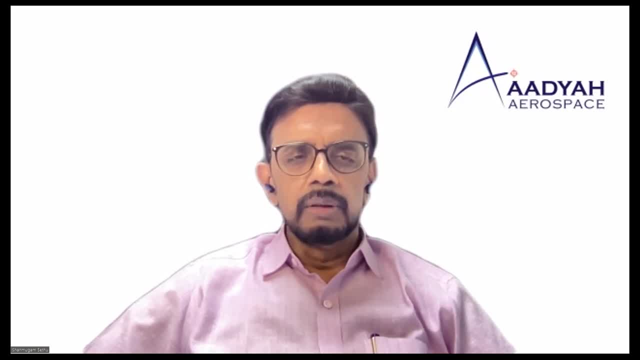 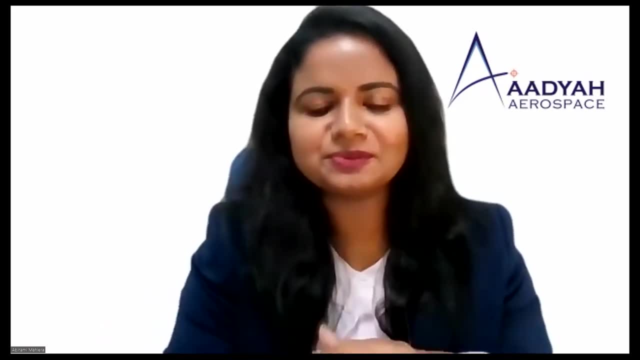 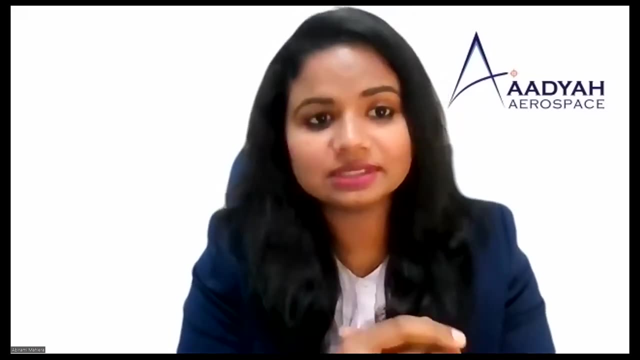 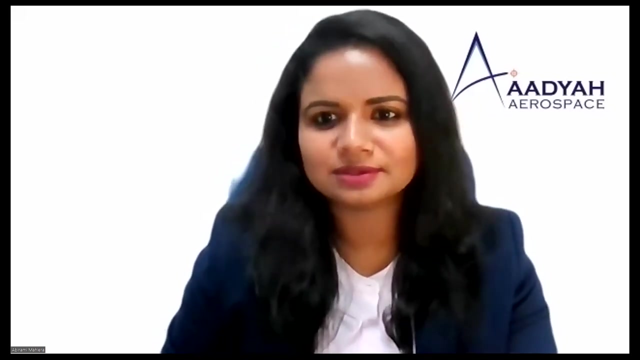 the processor and need to cater. you need to go in for the right sized processor. okay, um, so next we have another question from eshet. does shedding materials and the type of orbit have any relationship? and what about off the ship subsystems as well? let's check if eshet is online still, so that we can unmute him. 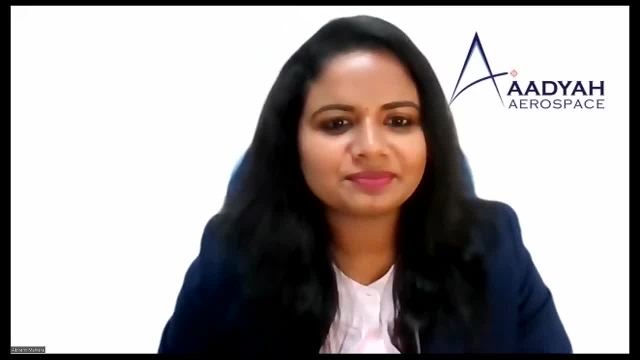 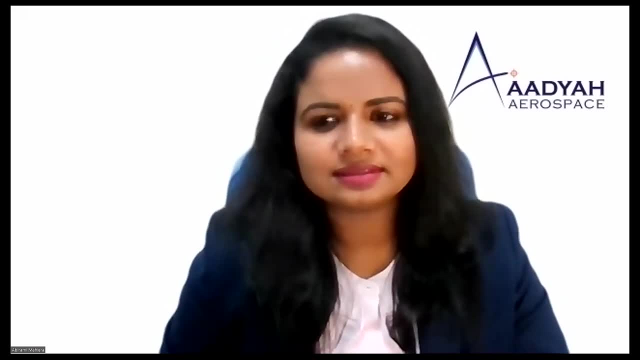 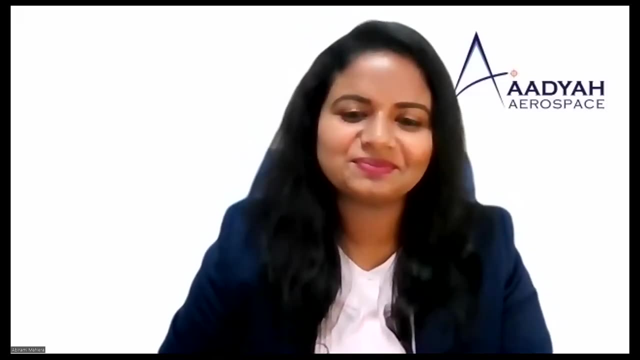 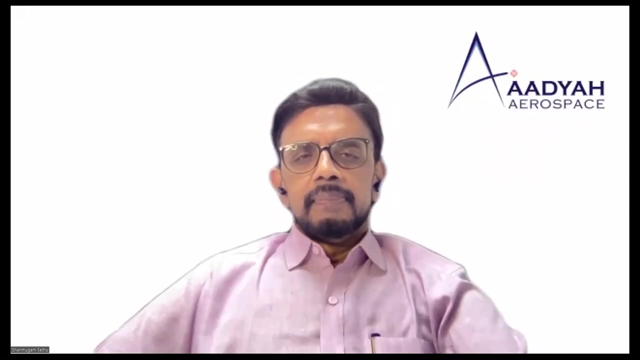 yes, please go ahead and have an introduction, okay. thank you for a nice presentation. thank you, okay. my question is regarding the shielding materials and the second is about of the shelf subsystems of satellite. the first is maybe, as we know we have, there are so many orbit. 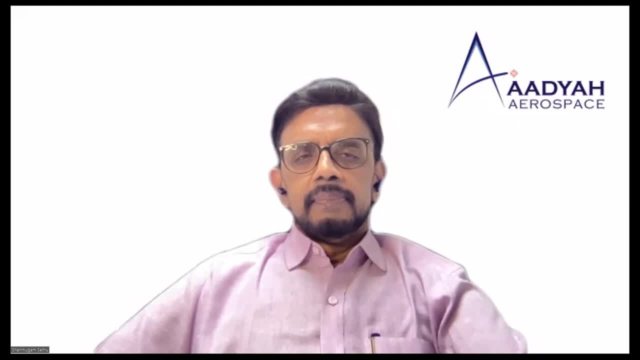 types of orbits, just like low orbit and higher orbits or geosynchronous orbits. something does the shielding materials have their own property depending on this orbits? the first question is this, and the second is about of the shelf materials. just recently, most of small satellites are already designed and most of them are of the shift from other materials. 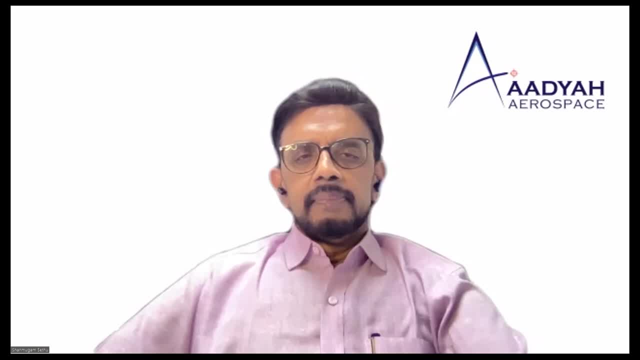 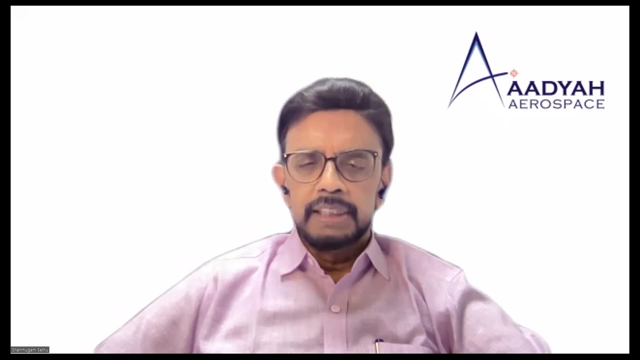 so is that any requirements to use this, of the shift materials depending on their orbits? absolutely, i think there is a orbit as a huge uh criticality with respect to the amount of radiation what the mission encounters. obviously, a lowest orbit will be a little bit uh lesser than, for example, the geosynchronous. 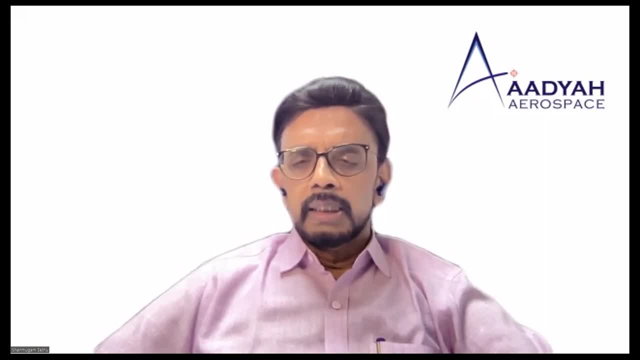 orbit at a higher point. that's it. so your initial uh radiation star evaluation will clearly tell you how much is the uh, the total ionization dose, expected during the mission and uh during the orbit of various cities of the orbit, and based on that you need to see whether. 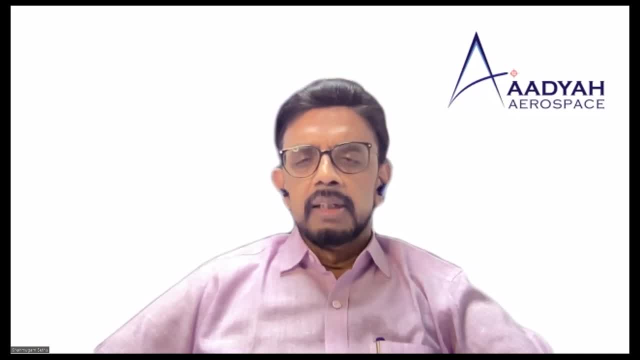 your electronics can withstand that. if it doesn't withstand the- suppose you have chosen your car's electronics- then the choice before you is that, whether you have, can build in the additional shielding material so that you can provide the protection now, uh, as you, as i was mentioning, to the 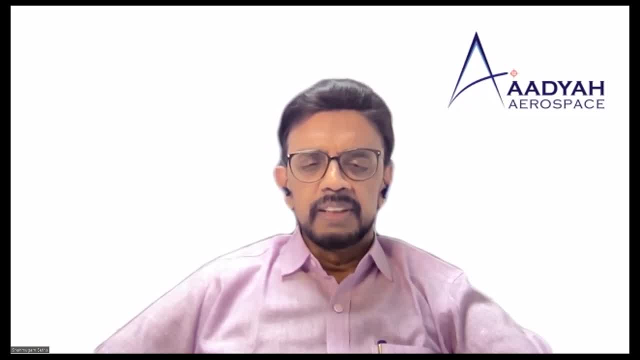 previous question. the choice of cars uh for uh cubesat or nanosat is uh pretty much uh wide varieties of the uh so wide uh numbers of car solutions available. but uh you need to carefully study how much of the radiation tolerance uh they have and whether it uh is less than the. 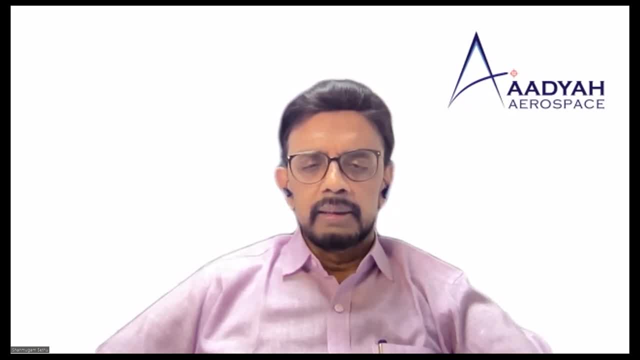 uh, or whether it is uh sorry, whether it's adequate or if it's less than the uh total ionization dose, so that you can take care of the total ionization dose what this uh, your radiation study, points out. so what? my immediate suggestion for you is that 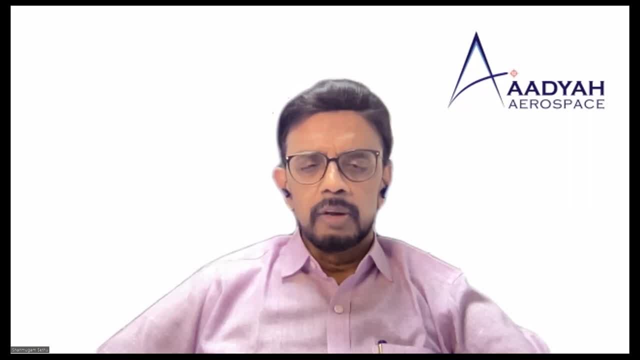 uh probably uh evaluation of the total ionization dose for the pacific orbit and then, followed by a good look at the what the radiation which your uh car solution can withstand, you may be able to decide upon the what needs to be uh corrective actions for your uh. 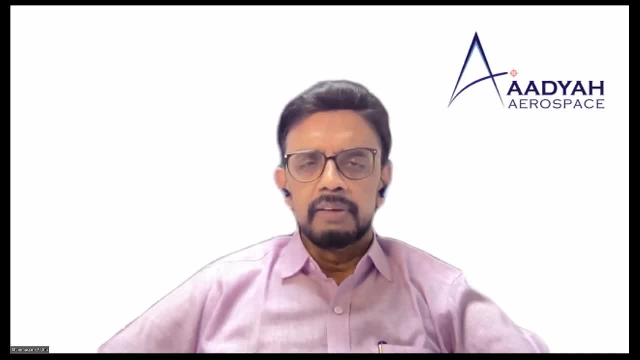 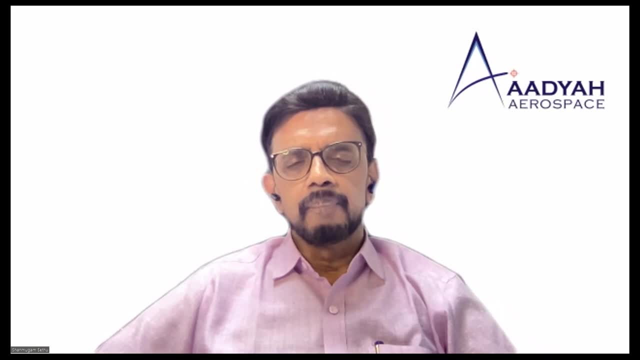 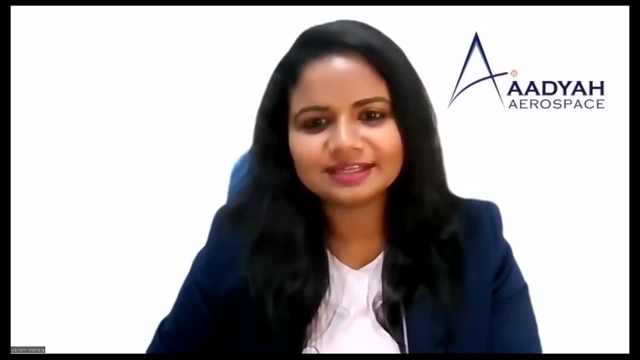 ensuring that the radiation doesn't affect the vision. does it test? answer your question? of course, yes, thank you, thank you. thank you, okay, thank you. we have another question from mr jane. he asks: what are coatings or finishes, avionics related devices that are outgassing resolute as well as having low magnetic susceptibility for space applications? 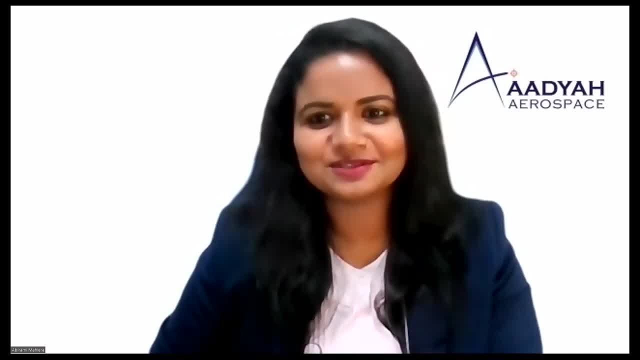 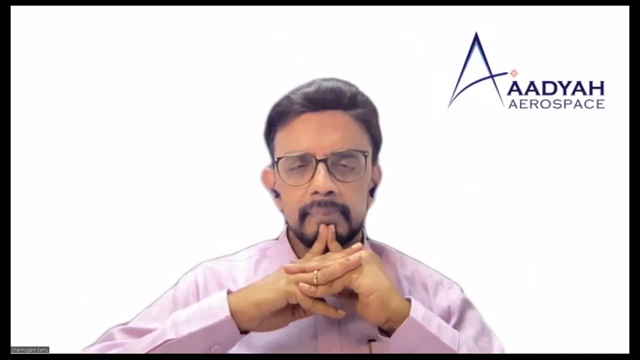 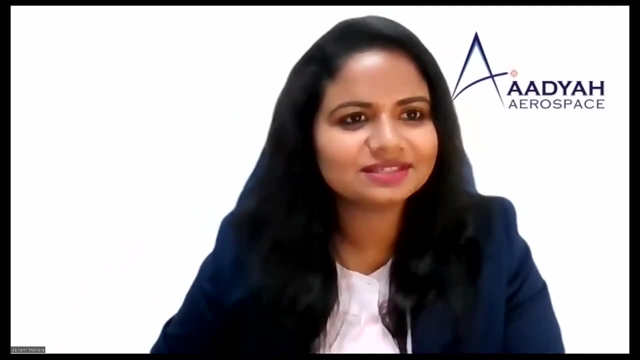 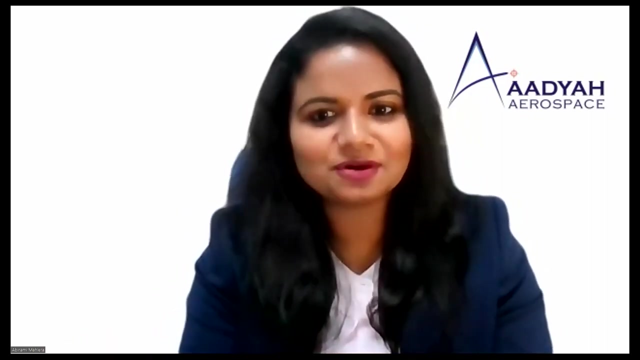 we would like to unmute james so that he can have an added interaction with you. oh, sure, looks like he has left. not an issue, please go ahead. mr sethu, do you want me to repeat the question again? yeah, probably i missed some portion of the question. um, so i think that, uh, he is asking: uh, what are coatings or finishes avionics? 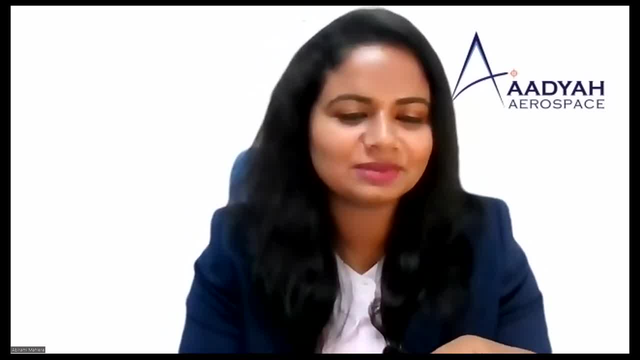 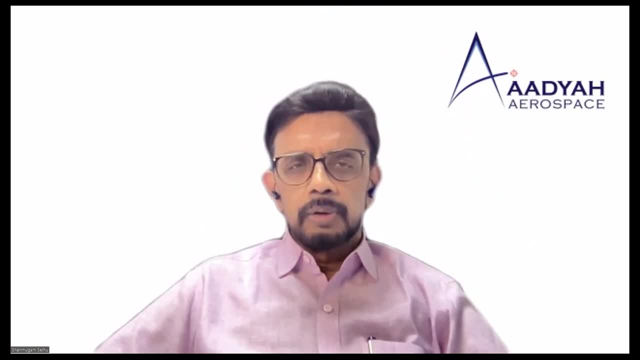 related devices that are outgassing resolute as well as having low magnetic susceptibility for space applications. so there are two portions of this question. is that uh? one is that he seems to require what are the low outgassing materials? and uh, the other portion is that, uh, he wants uh. 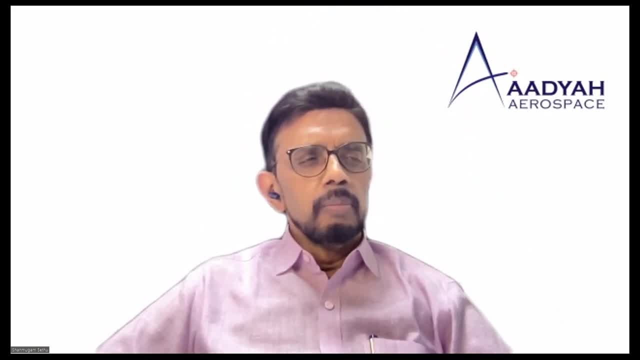 the same material to provide uh low magnetic susceptibility? i probably we need to. i'm making an assumption. here he is referring to the uh emi protection. i think so. to my knowledge, i don't think there is a material which can provide you both these advantages of uh. 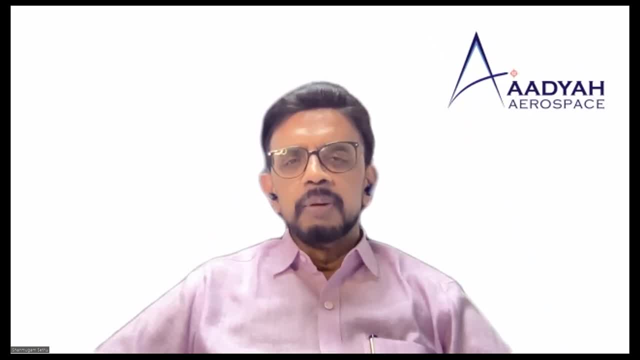 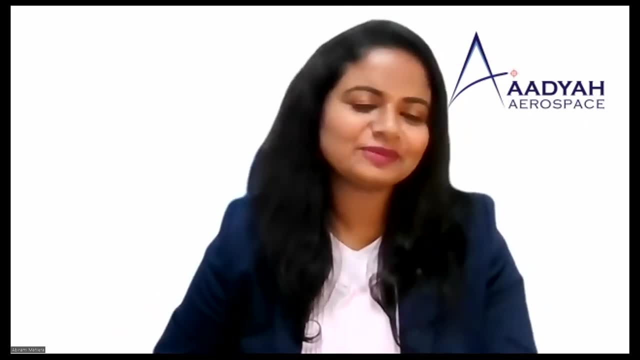 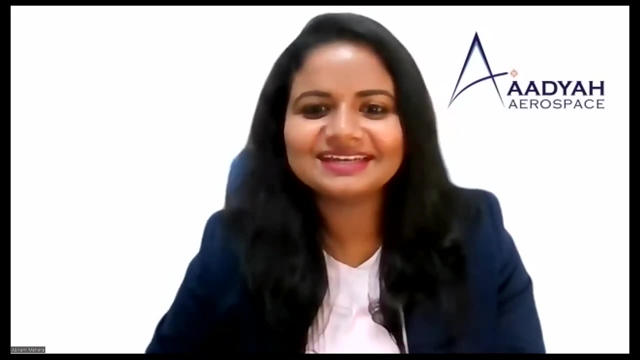 outgassing as well as the low magnetic things. probably we can get back to him if we have his uh cross okay, yeah, definitely we will try to get back to him on that. so one last question again from our our own anonymous attendee: is satellite affected with magnetic field distribution by? 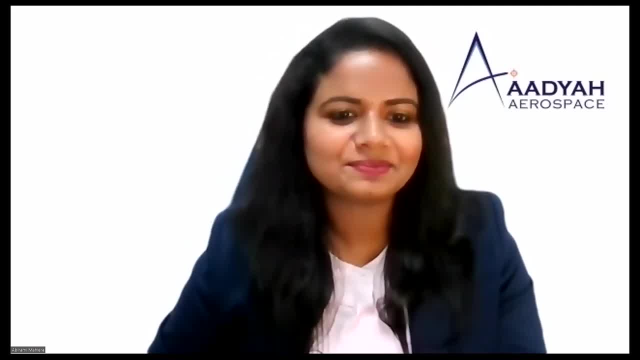 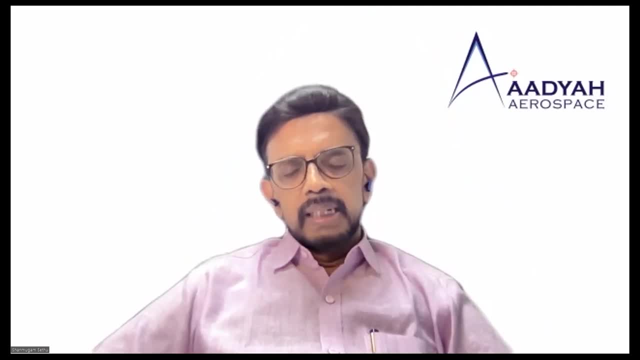 planets. how does it protect, okay, the uh once uh, the uh satellite affected by the magnitude uh? is that magnetic variation of the planet or the pull of the uh, or does it probably the question here refers to the uh gravity, i think. if i'm right, i don't know whether uh gravity magnetic has been used uh. 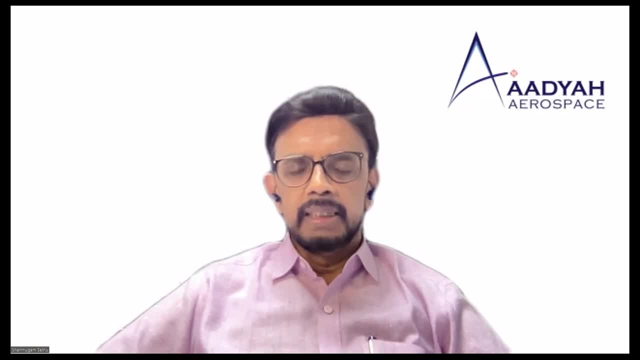 alternatively for the gravitation pull of the uh planets. now, uh yes, they do have a impact on your orbit. there are some uh well-known theory how an orbit can be altered in case of a magnetic or the gravitational pull radiations, or it can be altered by a slight disturbance in the 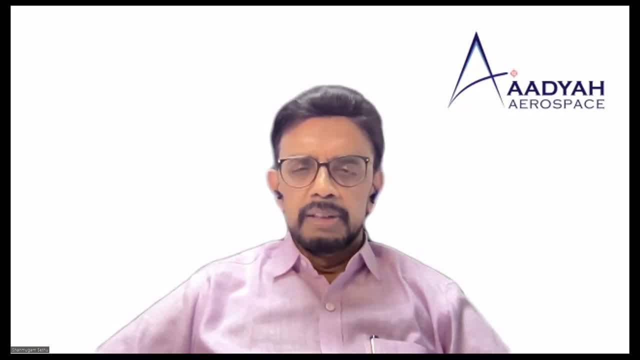 some of the outer solar system elements, etc. so there is definitely an impact, but thankfully, all of them are well researched upon and you have uh the what action need to be taken and that's where i think the uh orbital corrections, for uh that light comes in, because the 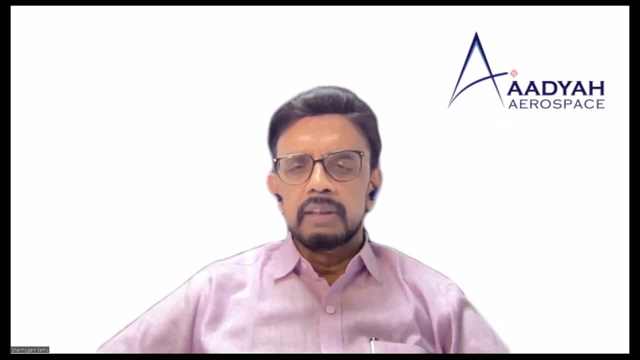 moment. uh, there, there are some deviations noticed, a significant one which will impact on the functioning or the mission of the satellite, and the orbital maneuvers are done to keep the satellite within the designated orbit. so, magnetic variations, field variations or, for that matter, your solar storms, or they also any amount of that. that's why a new topic is emerging, which is called as a. 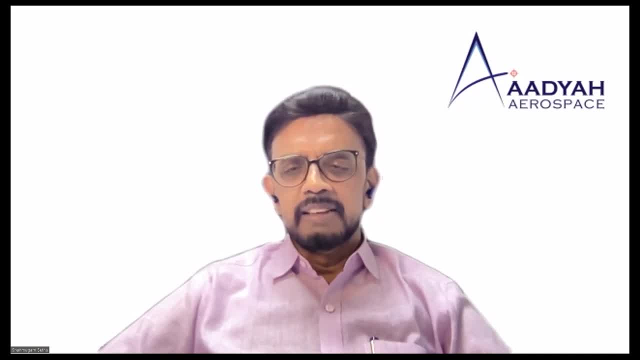 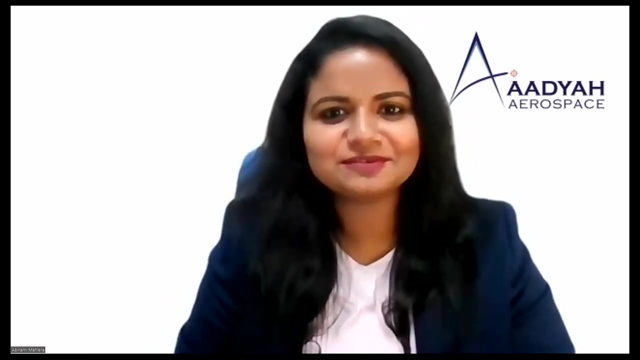 thezieh weather, where in uh, there is uh enough, uh enough, uh. signs that need to be created so that your mission doesn't get impacted to this weather or phase weather elements as such. okay, i hope that helps. all right, so we have the final question. this is from: